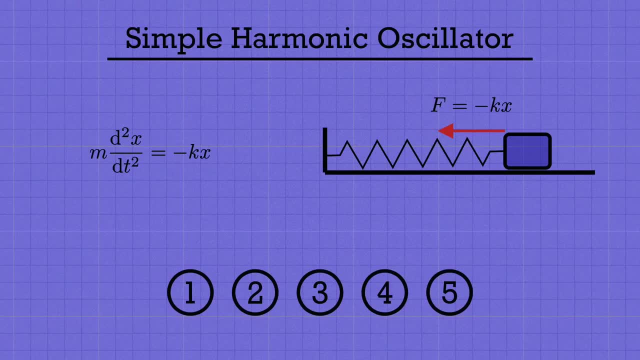 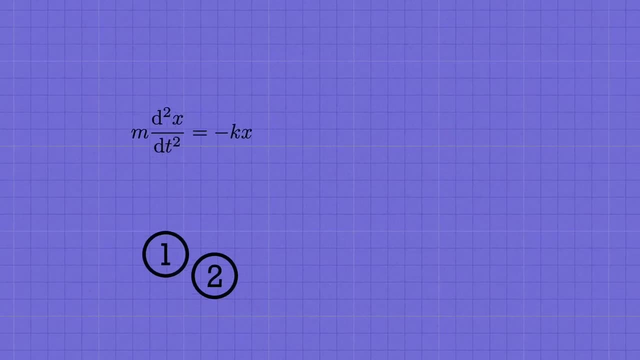 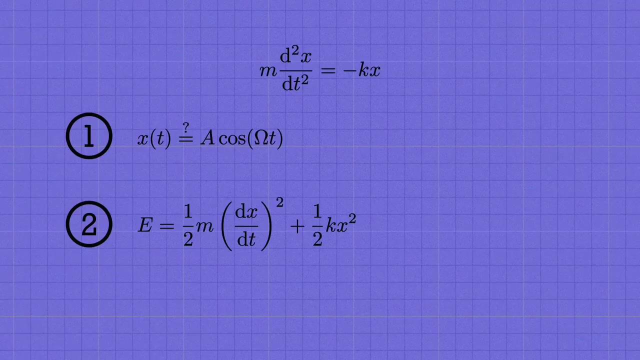 different about this video is that the five solution methods I'm going to show you will start from the most straightforward and work our way up through increasingly advanced approaches. So we'll start off seeing some relatively basic strategies for solving equations like this, which will already take you a long way, with lots of problems you'll meet in classical 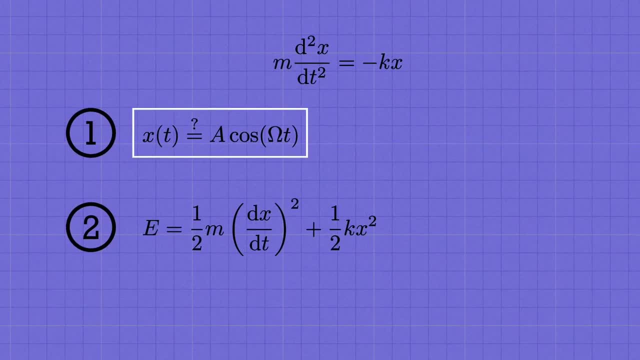 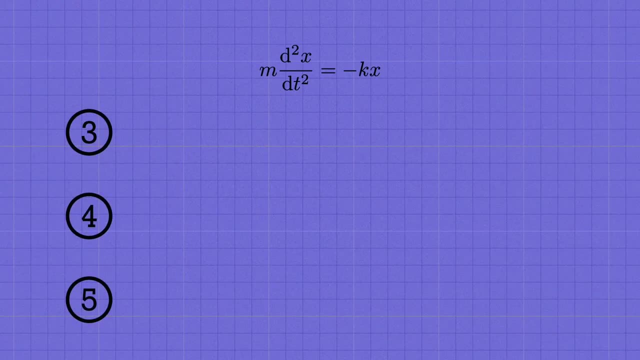 mechanics and beyond, like solving by making a substitution or using energy conservation. But as we go along, I'm going to introduce you to some more and more sophisticated techniques, like using a series expansion to solve the equation. using an integral transform, like 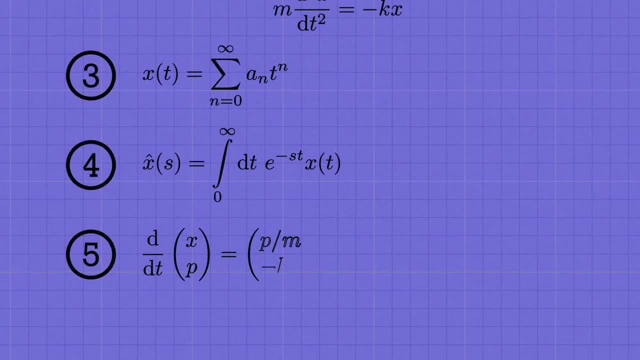 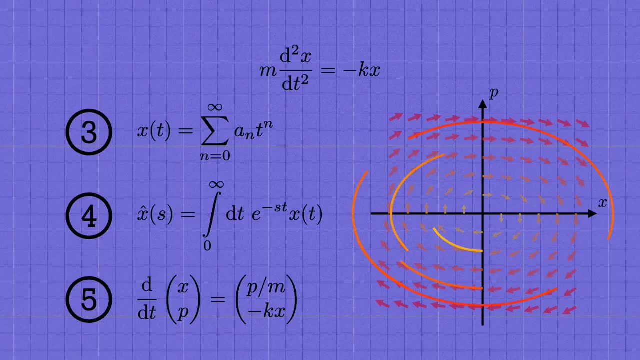 the Laplace transform. and finally, using Hamilton's equations, which also give us a new way of visualizing the solution as what's called a flow on phase space, And that's incredibly powerful. so make sure you stick around to the end to see that. 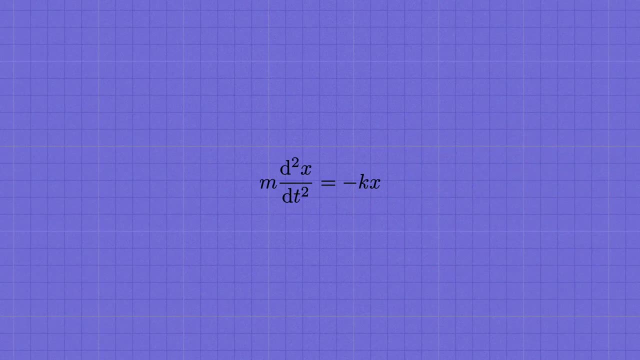 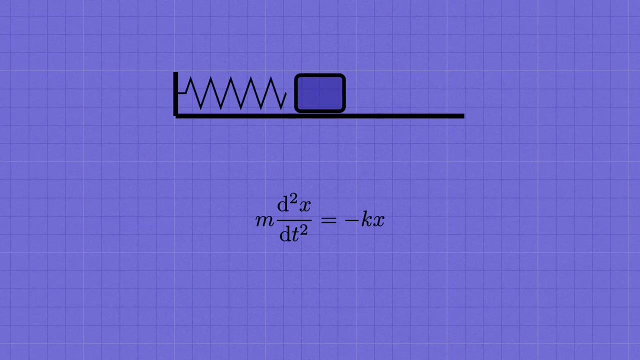 Okay, let's get going. First of all, let me quickly remind you where this differential equation comes from. Our setup is a block of mass m sitting on a frictionless table and hooked up to a spring of stiffness k In equilibrium. the spring isn't stretched. 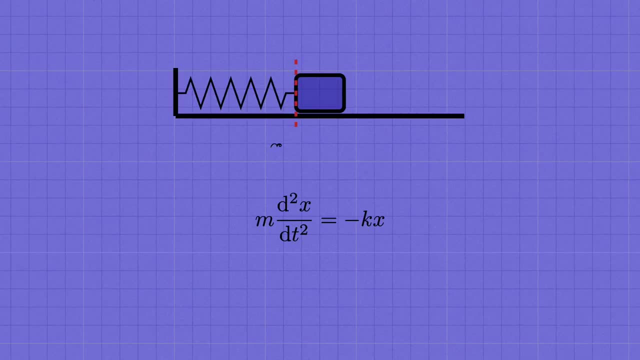 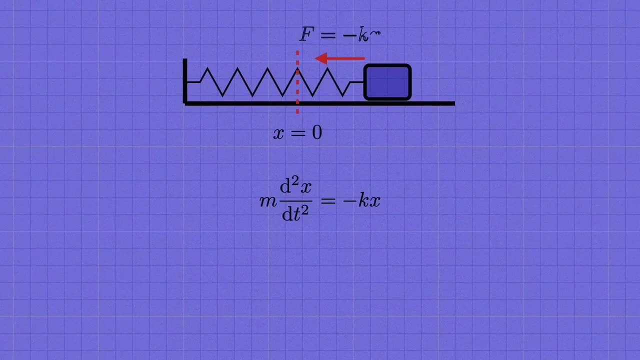 or compressed and the block can sit happily at rest there. Let's call that position. x equals zero. But if we slide the block away from there, the spring will now exert a force minus kx, trying to pull the block back toward equilibrium. Then the f equals ma equation. 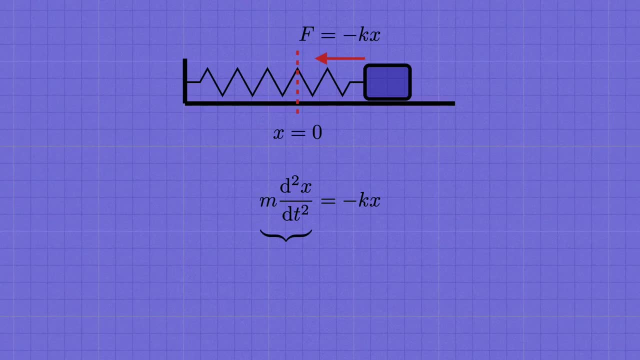 is simply m times the second derivative of x, that's the acceleration equals the force minus kx. Now let's say we pull the block out to an initial position, x sub zero, and then release it from rest. The stretched spring pulls the block back toward equilibrium, to the left. 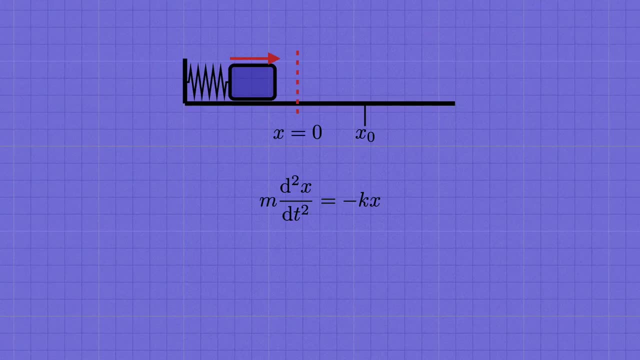 But then the block overshoots- x equals zero- and moves to the left of equilibrium. The spring gets compressed and pushes the block back toward the right, And on and on it goes, making the block oscillate back and forth around equilibrium forever. This is what we. 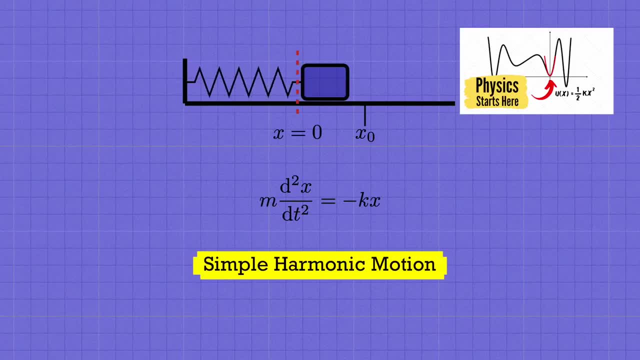 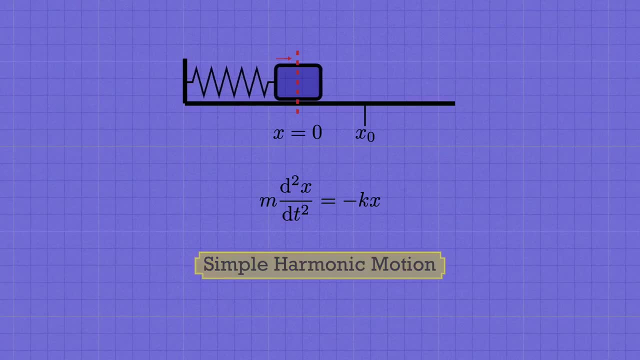 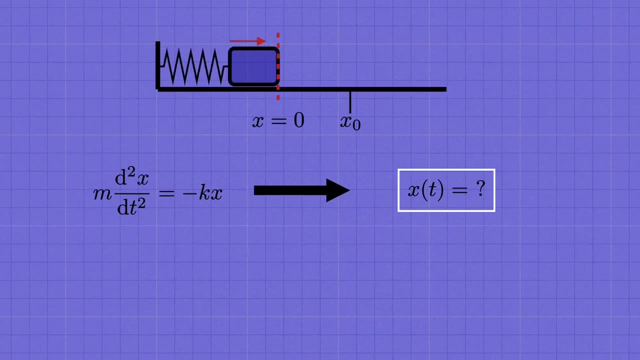 call simple harmonic motion. I made a separate video all about it, explaining why it's arguably the most important system in physics and why it shows up absolutely everywhere. But now let's see how to solve for the motion. from this equation We're looking for x, the position of the block as a function of time, And f equals. 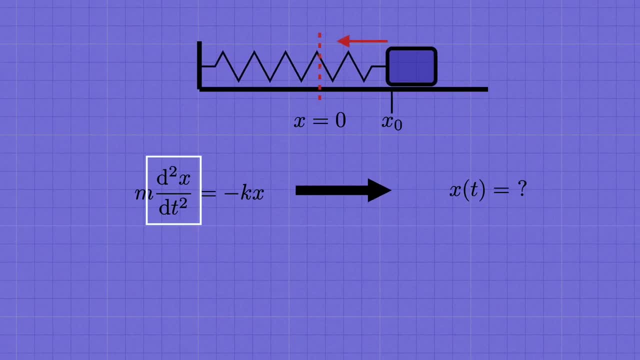 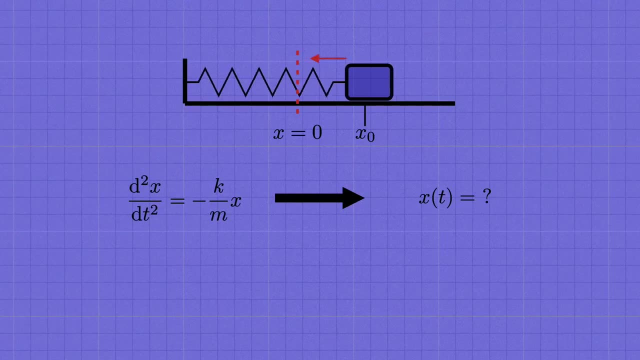 ma is a differential equation because it involves the derivatives of this function. It says that the second derivative of x with respect to t equals minus k over m times x again, And we're going to explore five increasingly advanced methods for solving this equation. 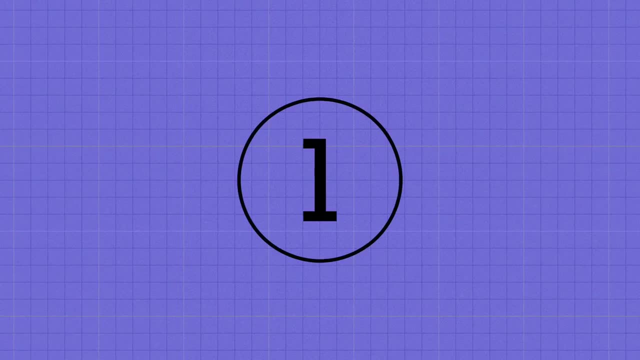 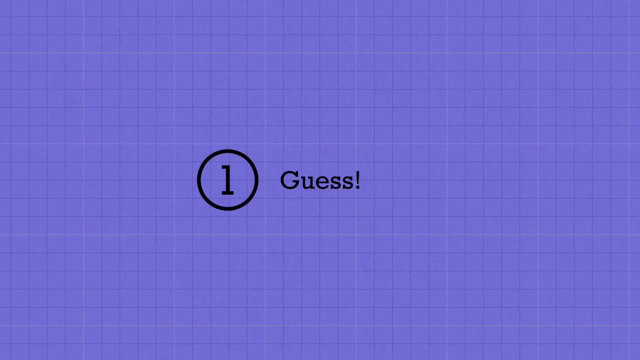 Starting off with number one, It might sound a little silly, but honestly, the first thing you can do, especially with a relatively simple looking equation like this one, is to try to guess the solution, Except that guessing doesn't sound very sophisticated. So instead, 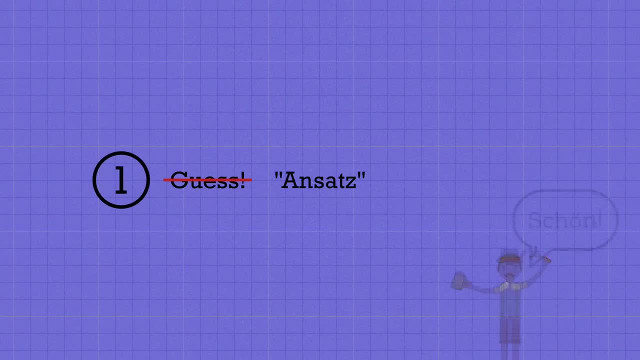 you'll often see textbooks call it making an ansatz, which is German and sounds much fancier. All that means in this case is that we're going to ask ourselves if we're going to solve this equation. First, we can think of a function which, when we take its derivative two times, we get back. 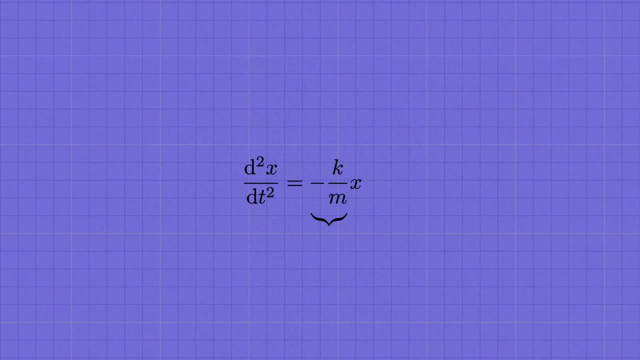 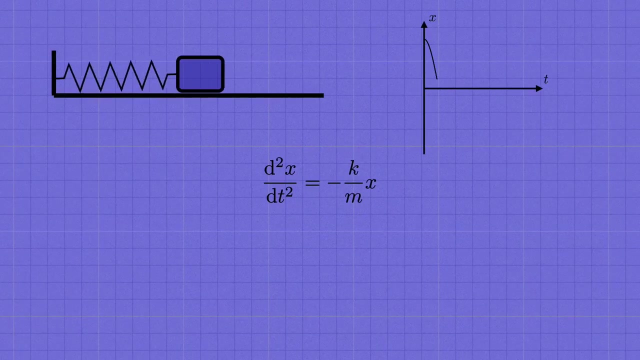 the same function. we started with times, some negative number. So what kind of function satisfies a property like that? Using our physical intuition, like we talked about before, that the block is going to oscillate back and forth around equilibrium, functions like sine and cosine might come to mind. 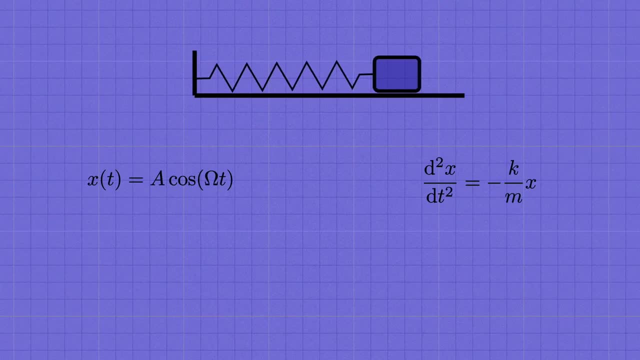 So let's make our ansatz and write down a guess of the form: a cosine, omega, t, where a and omega are some constants that we don't know the answer to. So let's make our ansatz and write down a guess of the form: a cosine, omega, t, where a and omega are some constants that we don't know the answer to. So let's make our ansatz and write down a guess of the form: a cosine, omega, t, where a and omega are some constants that we don't know the answer to. So let's make our ansatz and write down a guess of the form: a cosine, omega, t, where a and omega are some constants that we don't know the answer to. 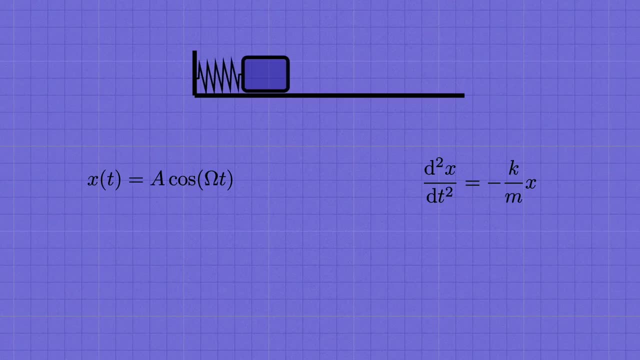 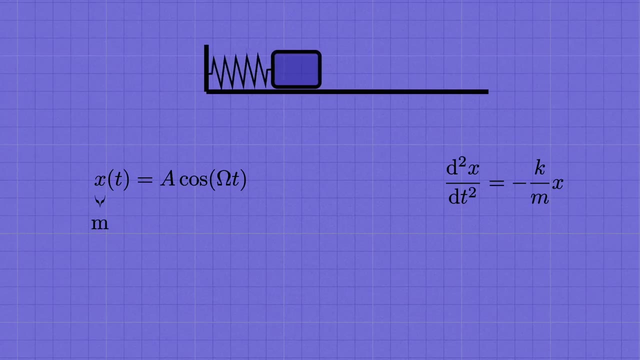 The idea is to see if we can choose them to solve the equation. We have to have some constants there just to get the units right. X is supposed to be a length, remember in meters say That means a. had better have units of meters too. 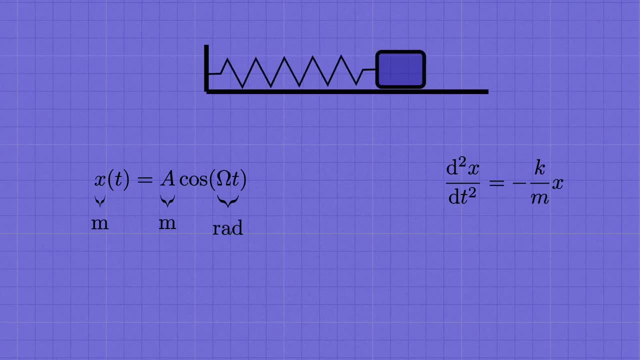 And inside the parentheses, omega t had better be measured in radians, which are dimensionless, So omega had better be something in radians per second in order to cancel out the seconds units from the t. Okay, well, let's substitute this guess into the equation. 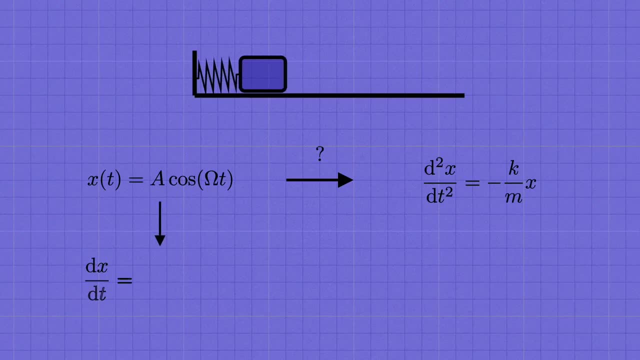 equation and see if it actually works. The derivative of cosine is minus sine and by the chain rule we also need to multiply by the derivative of the thing in parentheses with respect to t, which gives us a factor of omega. Now to do it again for the second. 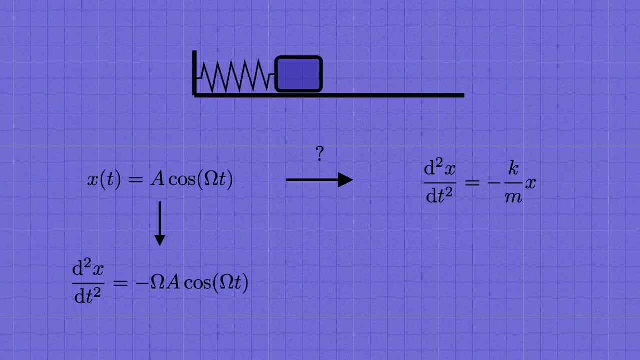 derivative. this time the derivative of sine is cosine, and again we get an extra factor of omega from the chain rule. Alright, that's what our guess gives us for the second derivative, But does it solve our differential equation? It looks promising because it says that the 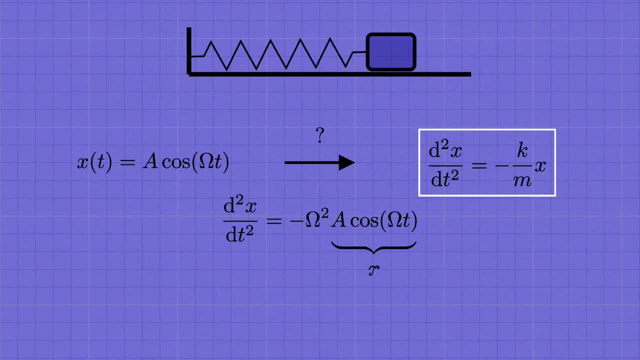 second derivative of x is indeed equal to x, again times a constant minus omega squared, Then all we need to do is pick this number, omega squared, to be the same as the ratio k over m that appeared in the differential equation, And that'll do it If we choose. 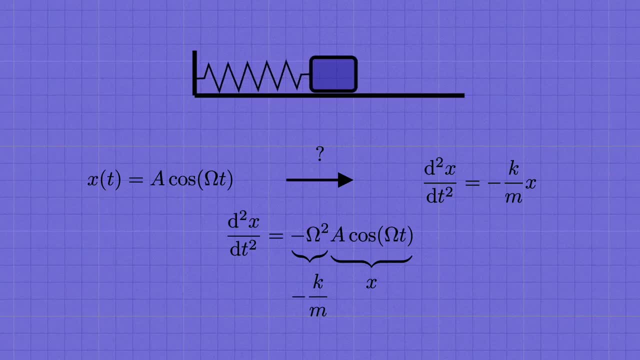 this value for omega, then x of t equals a cosine omega t will indeed satisfy the equation. So are we done? Well, no, First of all, sine of omega t satisfies this property just as well as cosine omega t, And so, more generally, we can add them together to write a general solution of this. 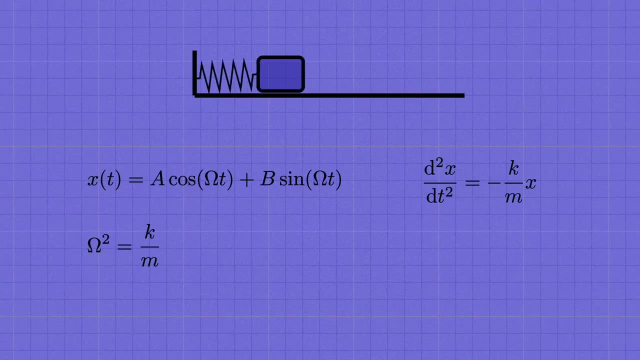 form That works because the differential equation is linear, meaning that we only have single powers of x and its derivatives showing up. But what are we supposed to do with these two constants a and b? This expression solves the equation for any values of these numbers. 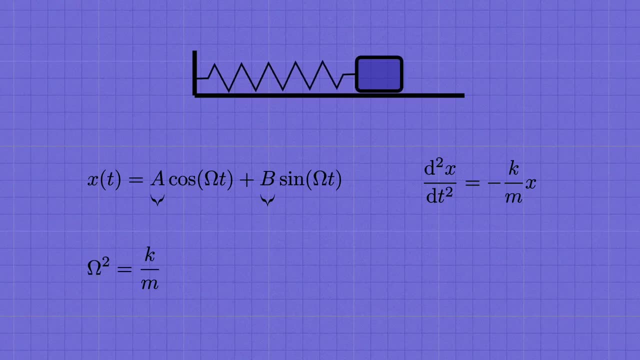 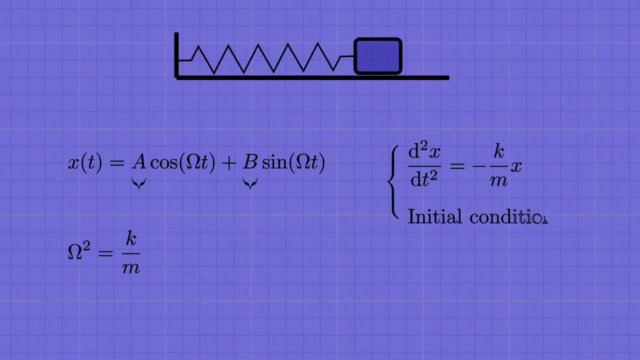 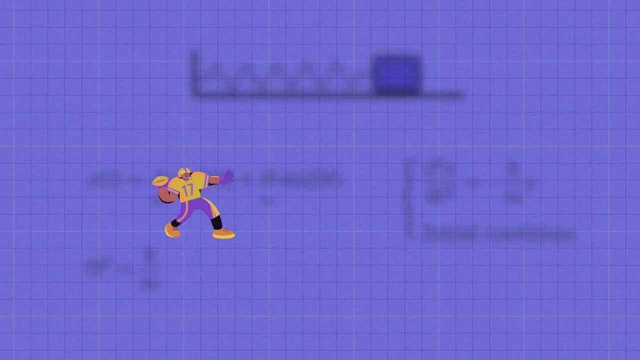 That brings us to a really important point about solving differential equations. The equation itself is only half the story. We also have to specify the initial conditions we want to satisfy in order to get the solution to the problem. Physically, that makes total sense. When you throw a ball up into the air, we need to know. 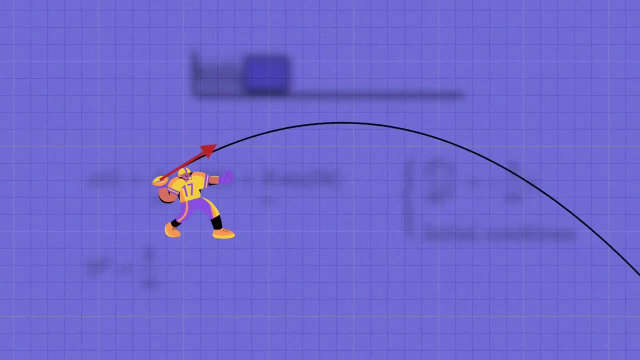 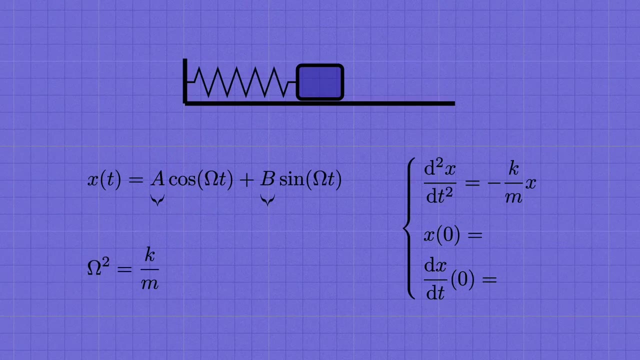 the initial position you're throwing it from and the initial velocity in order to be able to say what trajectory it's going to follow. Likewise, we need to know the initial position and the initial velocity of the block in order to say what its position will be after. 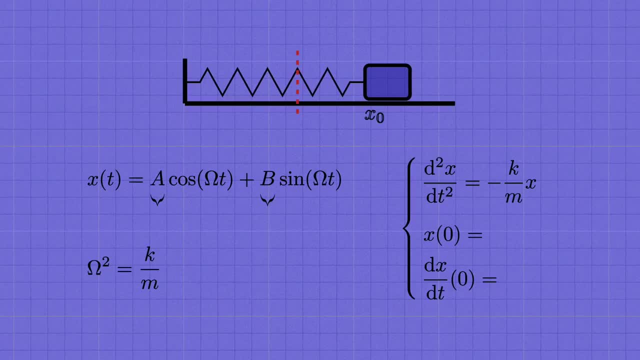 that In this case, we release the block from rest at x sub 0, and that means our two initial conditions are these: Mathematically, the fact that we need two initial conditions comes from the fact that the differential equation is second order, meaning that the highest 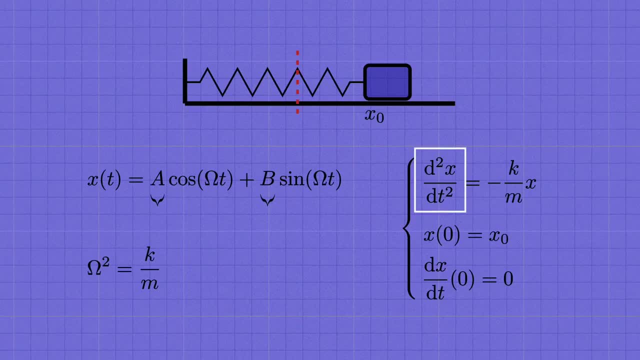 derivative that shows up is the second derivative of x. So when we plug in t equals 0, the sine disappears and cosine of 0 is equal to 1.. So now we have zero and cosine of 0 are equal to 1.. That means that the second derivative of x is the second derivative of x. So when 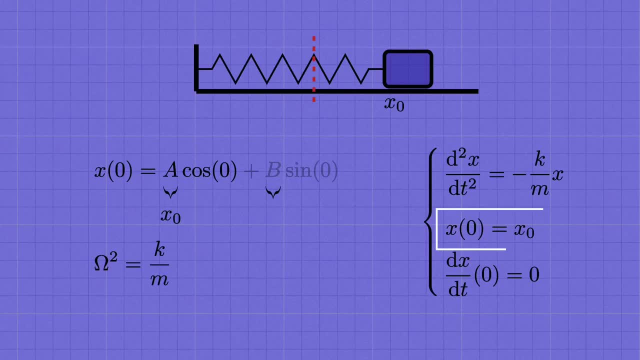 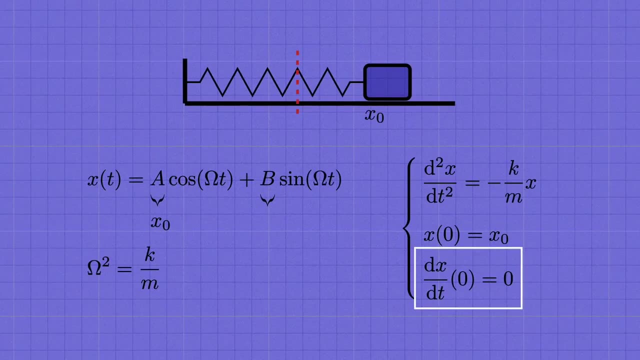 we plug in, t equals 0, the sine disappears and cosine of 0 is equal to 1.. We then have: So we'd better set a equal to x sub zero in order to solve our specific problem. Likewise, if you take the derivative and demand that the initial velocity vanishes, 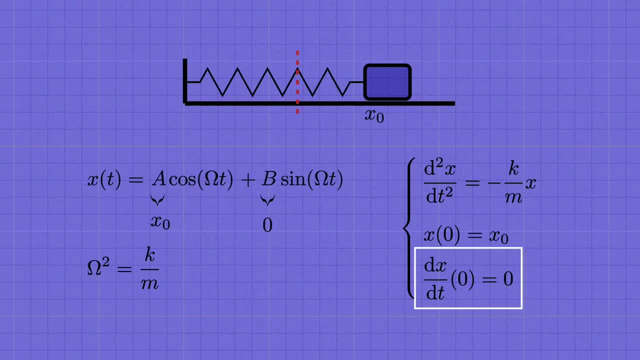 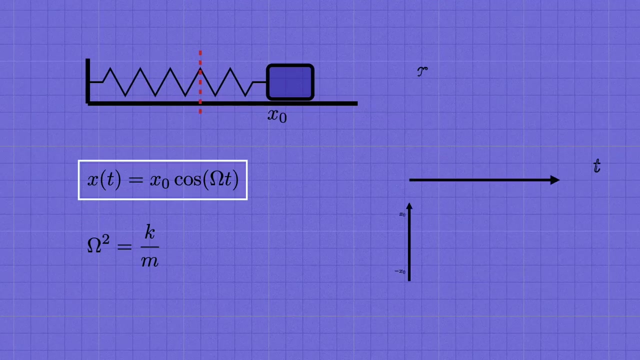 you'll see that we need to set b equal to zero, And that leaves us with x of t equals x sub zero cosine omega t, where again omega equals the square root of k over m, is fixed by the stiffness of the spring and the mass of the block. This looks about like we'd expect: The block starts. 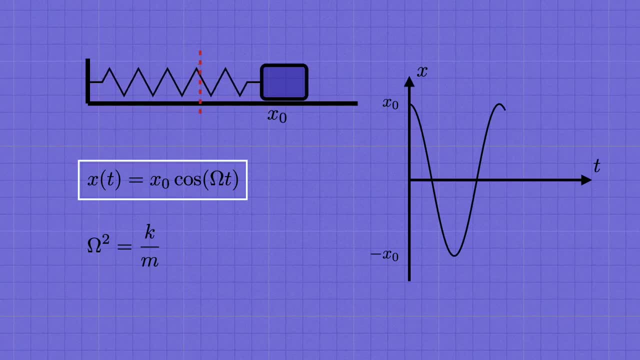 out at rest at the initial displacement x sub zero, and then, when we let it go, it oscillates back and forth around equilibrium, where omega controls how fast it oscillates. So there we have it. We've solved the differential equation, together with the initial conditions. 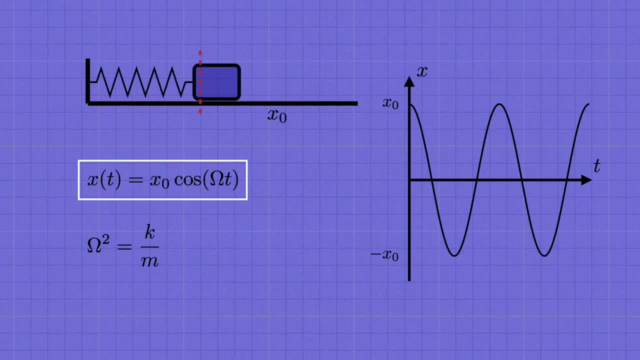 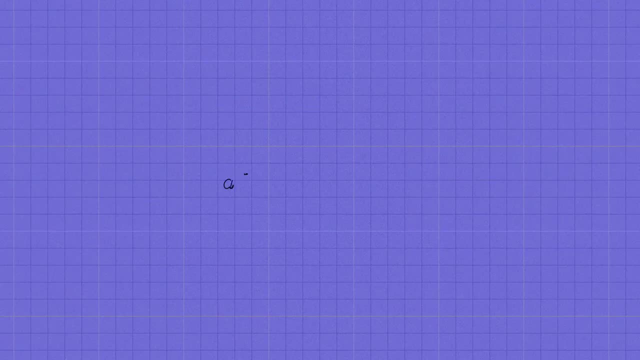 by substituting in a guess or ansatz with some constants in it and seeing how to pick the constants in order to get a solution. And this kind of strategy works in general for a linear equation like this, where a, b and c are some constants. 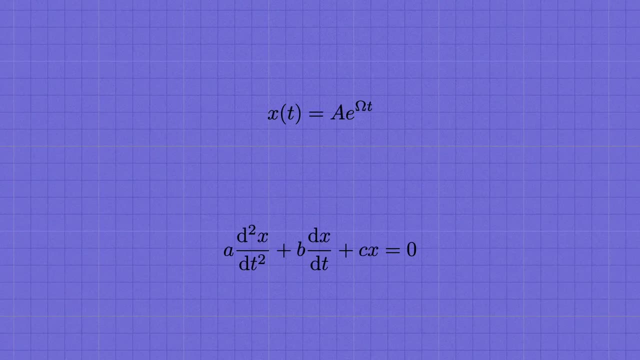 In general, you'd pick an exponential for your guess, a e to the omega t, substitute it in and see what conditions come out on those constants. Explaining that whole method in detail, though, would really deserve its own video. For now, we're going to stick with the simple harmonic oscillator equation. 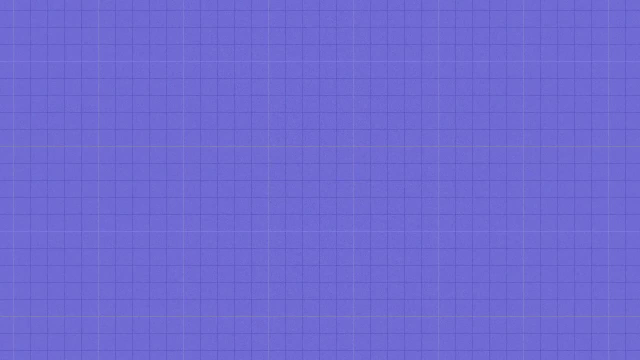 and see four other really powerful ways of approaching it. And that brings us to method number two: using energy conservation to solve the equation. As you've hopefully learned before, if we take the kinetic energy of the block- one half m times the velocity squared- and add to it the potential energy in the spring, 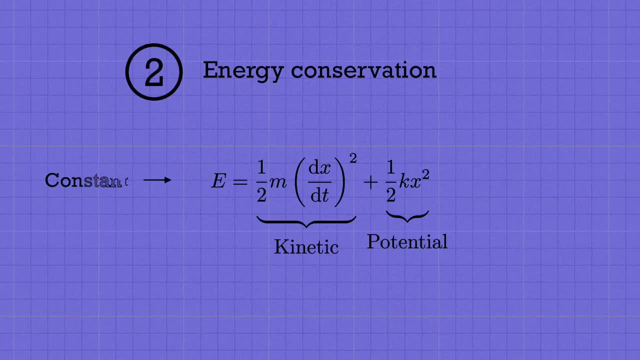 one half k x squared, we'll get a constant: the total energy. That's not obvious because both x and dx by dt are changing with time as the block slides back and forth. But when we add them together in this special combination, 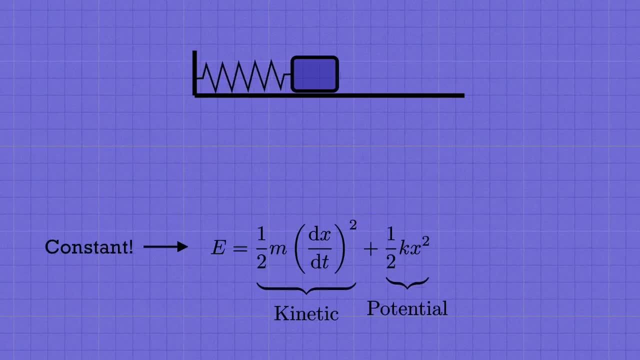 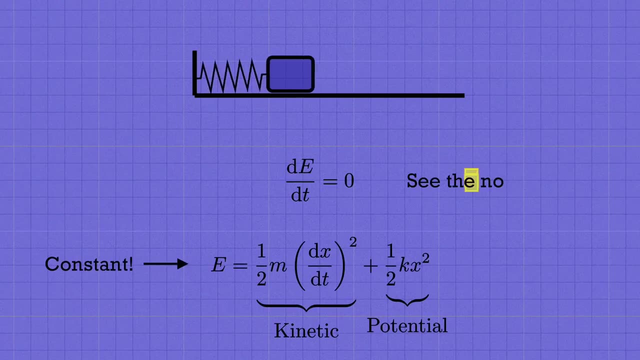 the t's drop out and we get a constant. The way to check that that's true is to take the derivative of e with respect to t and see that it's equal to zero. I'll show you how to do this. I'll show you how to prove that in the notes which you can get at the link in the description. 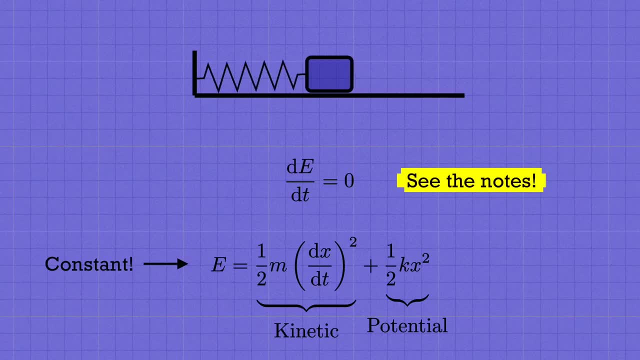 and where I'll go through everything we're covering in this video in more detail. If you really want to learn all these concepts, you should watch first to get the general idea of how things work and then go through the notes to take your time processing the material. 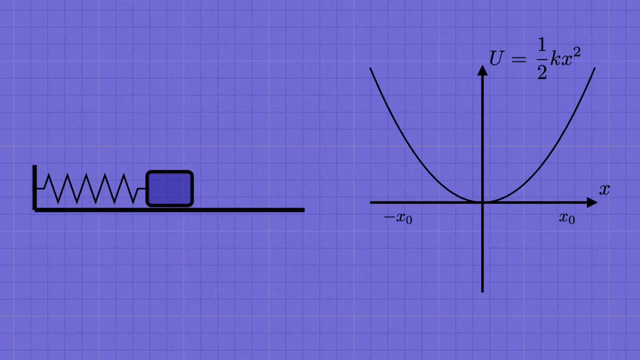 In this case the potential energy is a parabola. So when we release the block somewhere over here at x sub zero, all of the energy is the potential energy stored. in the spring There's no kinetic energy because we're releasing the block from rest. Then, when we let it go, the block starts to speed up. 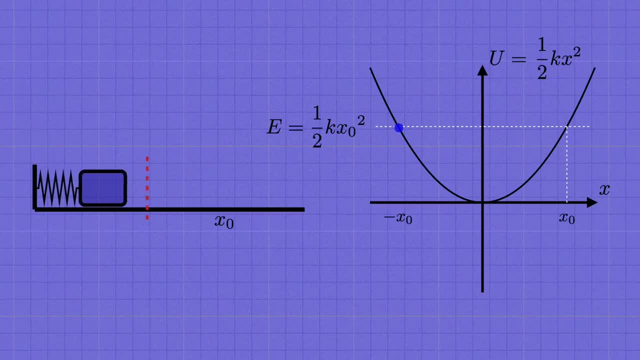 and the spring starts to relax. By the time it reaches, x equals zero. all the energy is kinetic, and on and on. the energy cycles back and forth between kinetic and potential, But the total energy never changes. It's always the same number. we started with 1 half k, x, sub. 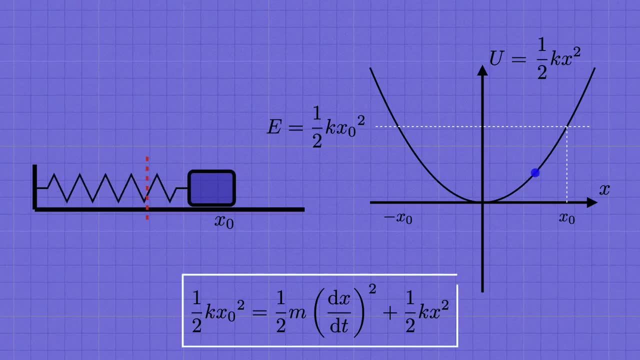 zero squared, And what we'll see now is that we can use this equation for energy conservation to solve for the trajectory of the block. It's again a differential equation for x, but notice that it only involves the first derivative of x, not the second derivative that we had in. f equals ma. 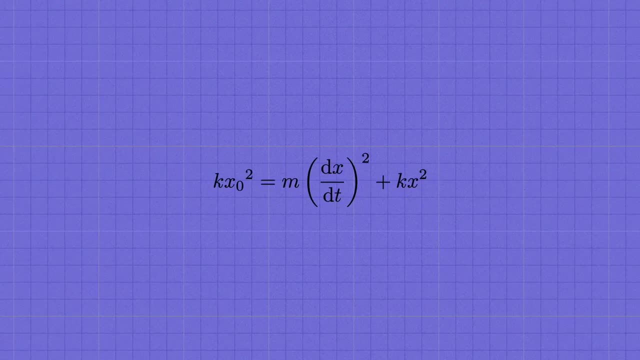 Let's rearrange the equation a bit. We can cross out the halves, and I'll also move the k- x squared over to the left hand side and then divide by m. I'll also use the same symbol, omega squared as before, for the ratio k over m. 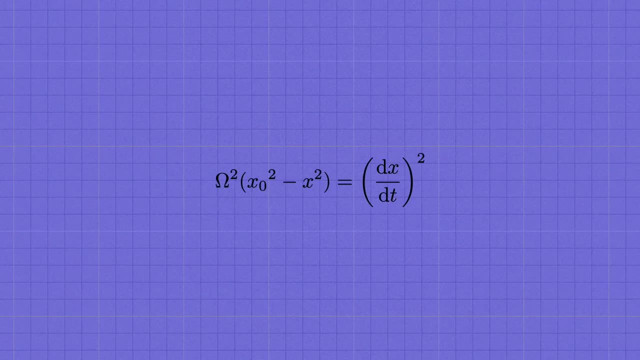 Remember, omega was what told us how fast the block would oscillate back and forth. And finally we can take the square root to get an equation for dx by dt. Now something really special has happened. This equation tells us the velocity of the block. 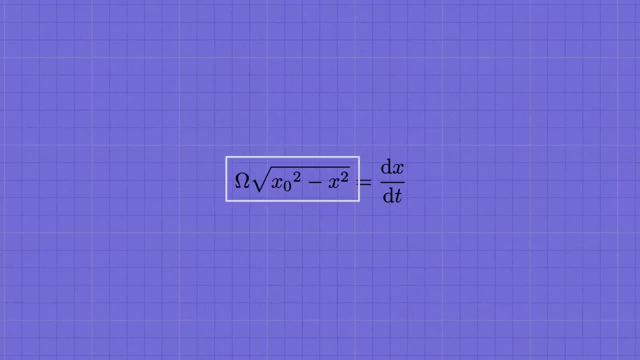 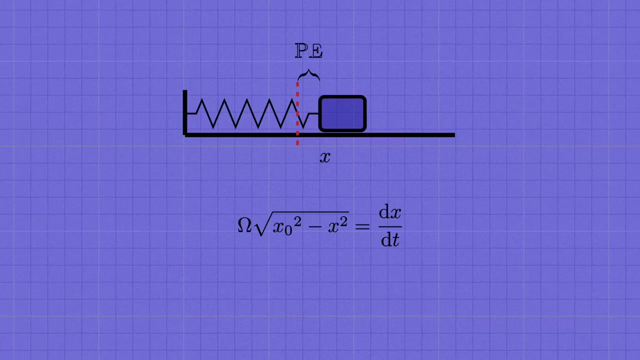 as a function of its position x. The point is, if we know the position of the block, we know how stretched or compressed the spring is and therefore how much potential energy is stored in it. Then conservation of the total energy tells us how much is left over for the kinetic. 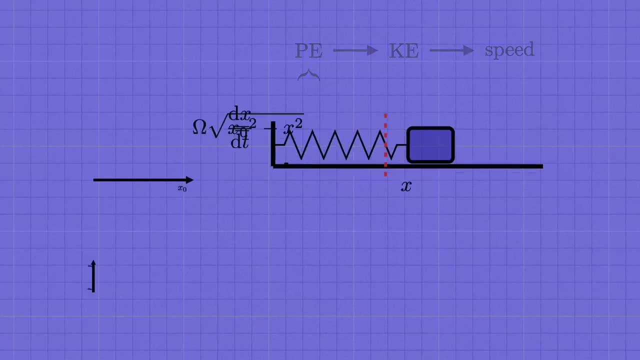 energy of the block And that's the final result. And finally, we can take the square root to get an equation for the velocity of the block and therefore how fast it's moving. So when the block starts off at x sub zero, we get v equals zero, because we released it from rest. 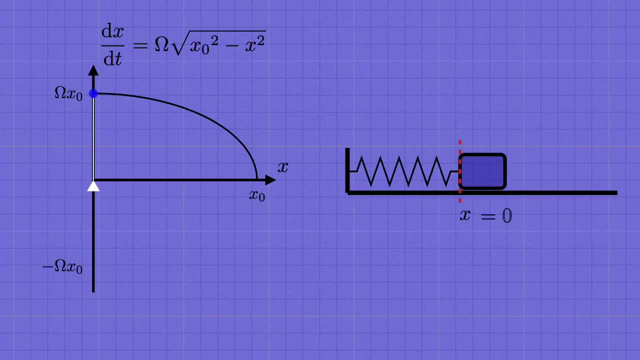 But by the time the spring pulls the block back to equilibrium at x equals zero, it's sped up to its maximum velocity and we get dx by dt equals omega times x zero. Actually, we should really get minus that, because the block is initially moving to the left. 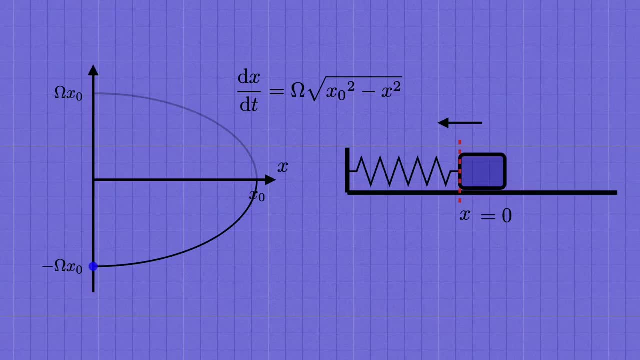 So we ought to be a little more careful when we take the square root, since we can get either sine. We take the minus sign when the block is moving to the left and the plus sign when it turns around and goes back to the right. And now we can solve for x of t by integrating one more time. 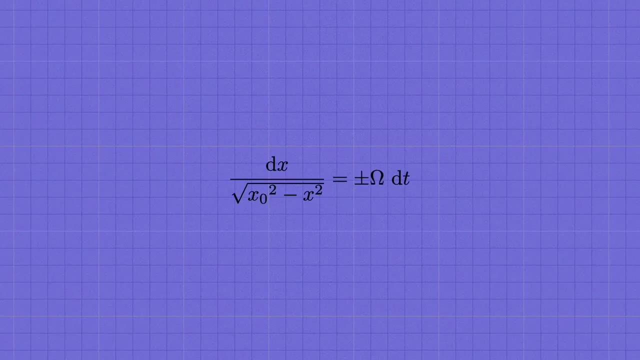 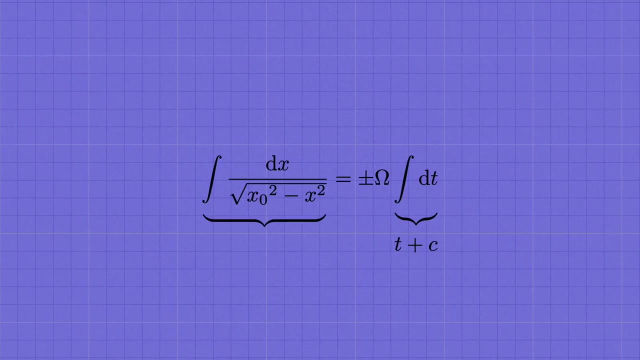 Just divide the square root over to the left hand side and multiply the dt over to the right in order to separate the variables. Next we integrate both sides of this equation. The integral on the right is super easy. We just get t, maybe plus some integration, constant c. The integral over x is a little harder. 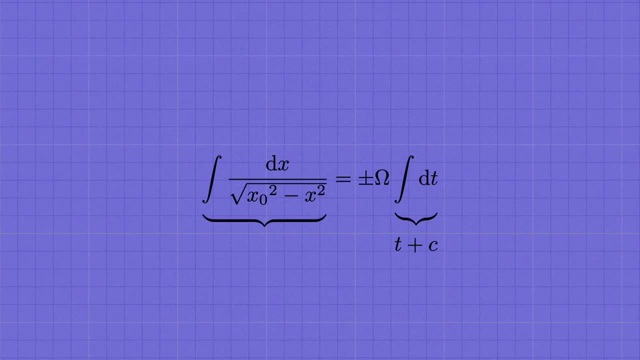 you can do it with a trig substitution or of course you can just look it up. It's given by minus the inverse cosine of x over x zero. We could also add another integration constant here, but we can just absorb that into the other constant c on the right. Now we solve for x. 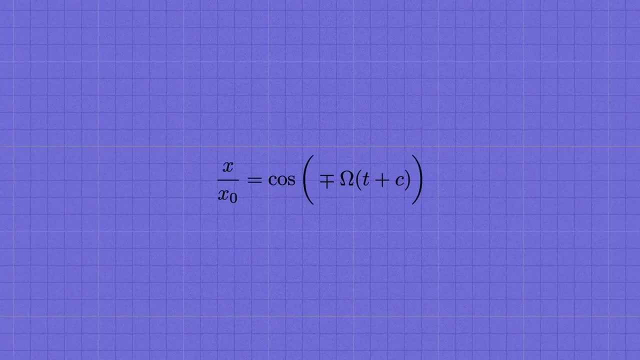 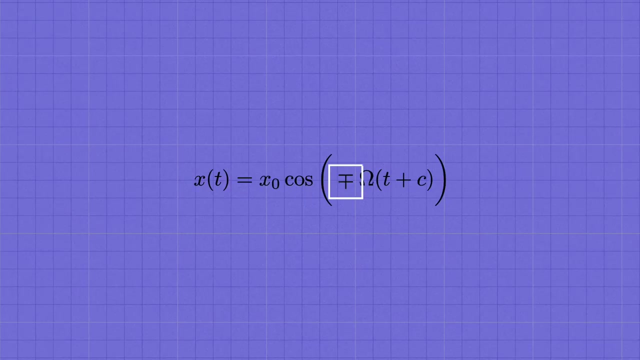 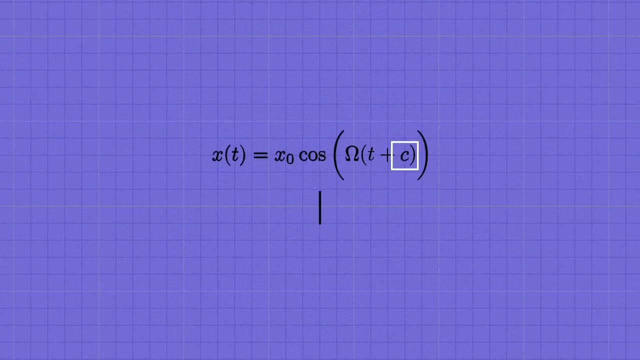 Flip the sine, take the cosine of both sides and move the x- zero over to the right. Now we're almost there. Cosine doesn't care if you plug in plus or minus something, it's an even function. So we can throw out the plus or minus. And as for the c, remember that when we plug in, t equals zero. 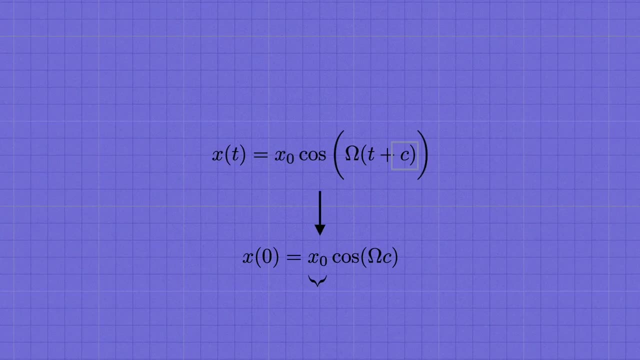 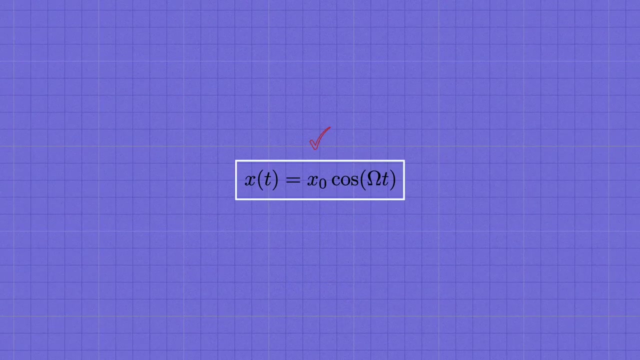 we want to get x sub zero, So we can just set c equal to zero. Then at last we get x of t equals x sub zero, cosine, omega t, just like we found with method number one. So conservation of energy also lets us easily get to the solution of our differential equation, And in fact this: 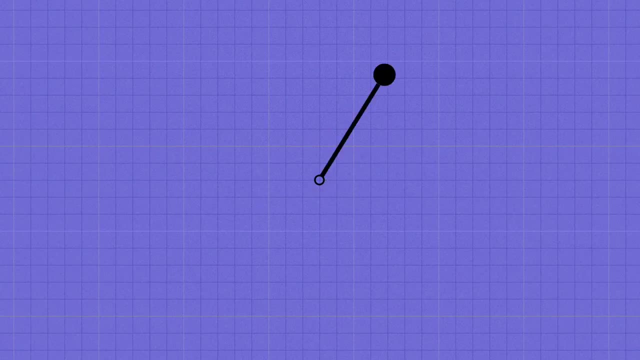 strategy can often be successful for harder problems, even when our first method wouldn't work. A great example is the simple pendulum, which is supposed to be so simple that it's in the name, but actually it's surprisingly tricky. I'll let you play with that one for yourself, for practice. 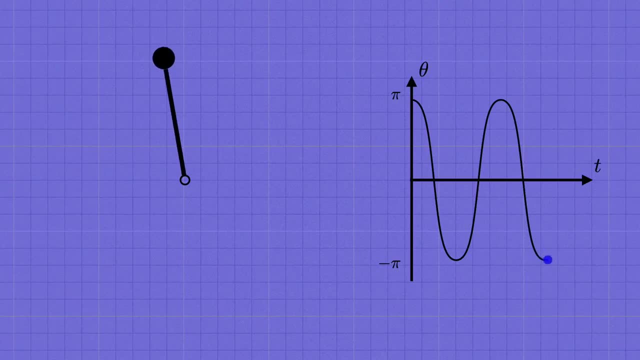 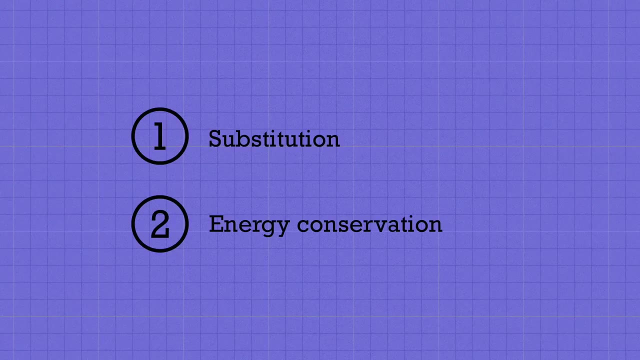 with this method and I'll share some more details about it in the notes. So now we've seen two different ways of solving the harmonic oscillator equation, and these will more or less do the job. for most of the equations you'll meet in your first mechanics class, But if you're up for it, 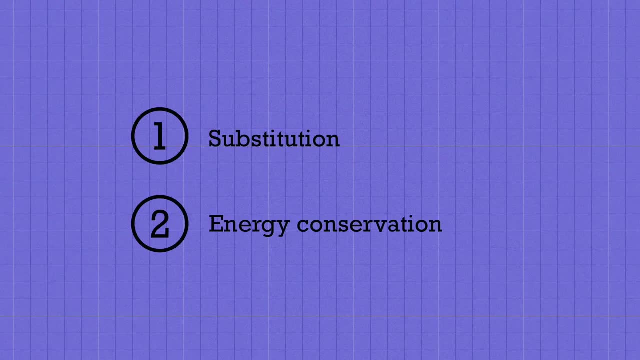 what I'd like to do now is show you some more powerful methods that will come in handy later on, when you're faced with harder equations. So let's plow ahead to method number three, using a series expansion. This one is probably the most versatile of all the strategies we'll see here. 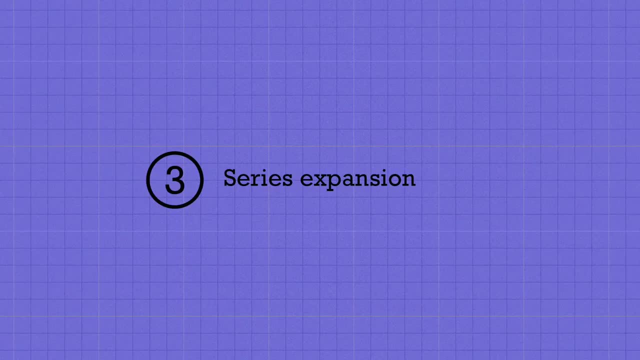 and you can apply it to most any differential equation to get an exact or even just an approximate solution. The idea is, whatever the solution x of t to our differential equation might be, we can almost always expand it as a Taylor series in powers of t. 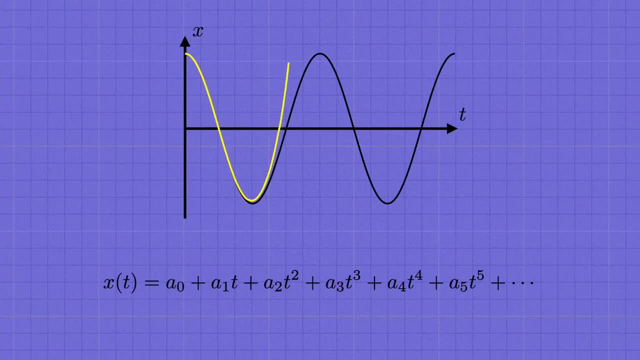 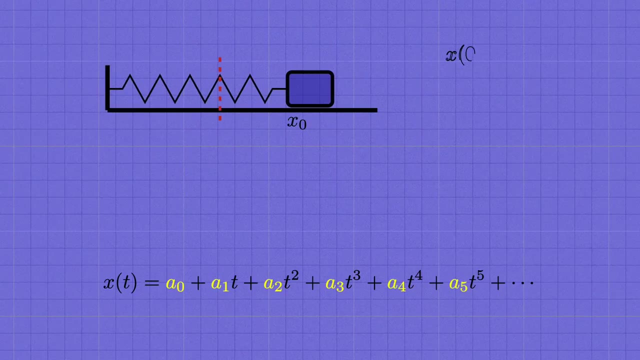 at least within a window where things are well behaved. The question is, how do we figure out these coefficients are supposed to be Well, first of all, let's go ahead and impose our initial conditions. When we plug in, t equals zero to the series expansion. all the t's disappear. 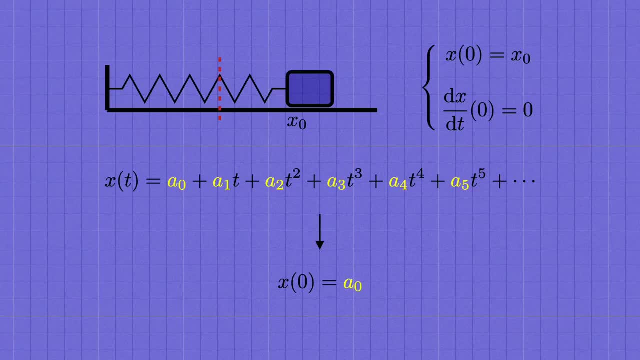 and we're left with x of zero equals a sub zero. So we want to set that equal to x zero to coincide with the initial position of the block And to impose that the initial velocity is zero. we'll take the derivative of the series a one plus two, a two times t plus three, a three t squared. 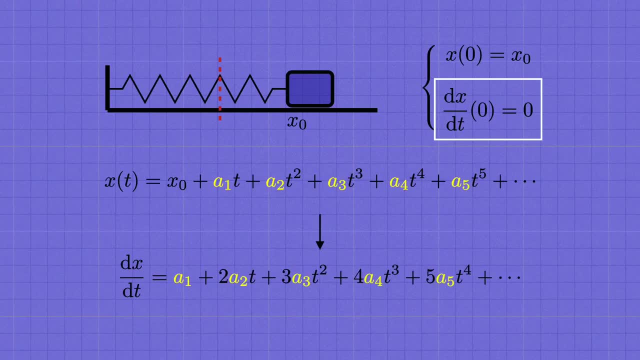 and so on. Now, when we plug in t equals zero, we're left with a sub one, And so we want to set that equal to zero. All right, so far we figured out a sub zero and a sub one, But there are still. 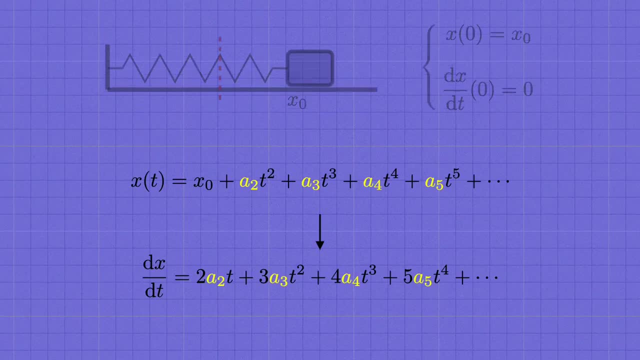 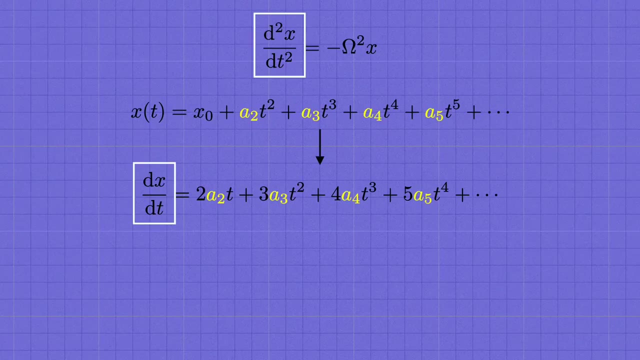 infinitely many coefficients left to determine. So the next thing we need to do is actually plug the expansion into the differential equation. That means we need to take the derivative of the series one more time to get the acceleration we'll have two times a two plus three times two. 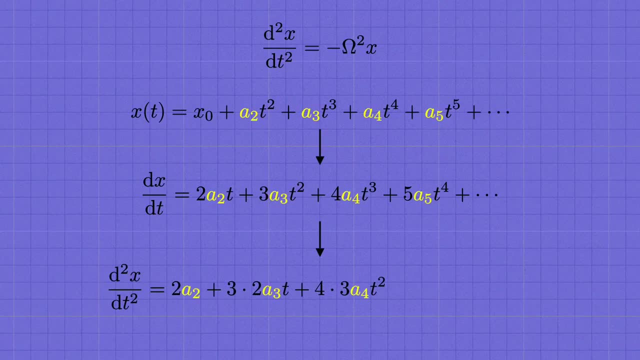 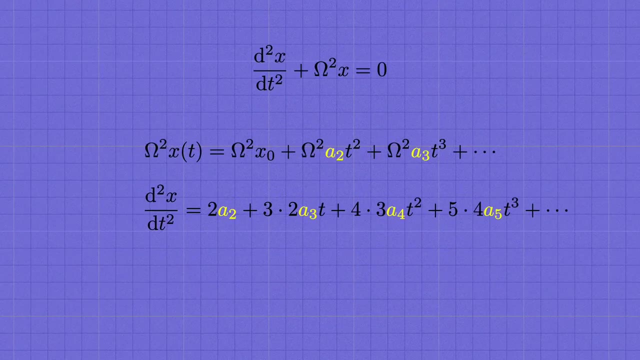 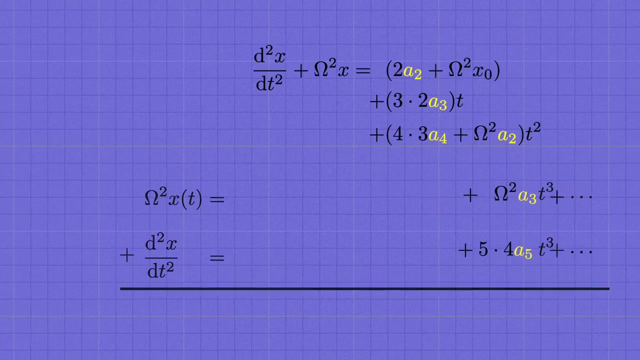 a three t plus four times three, a four t squared and so on. And now we add on omega squared times x, and set the whole thing equal to zero, And it's helpful to pair up the corresponding terms. All of this needs to vanish if we want our series to solve the differential equation. 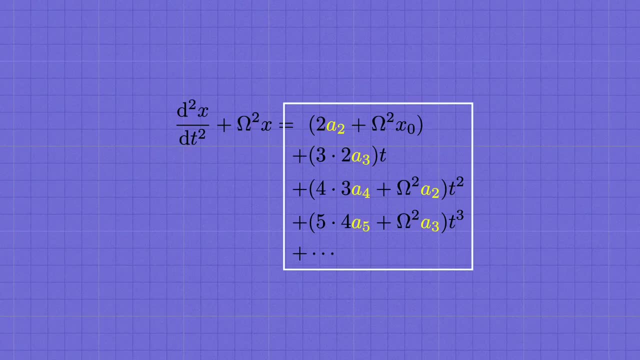 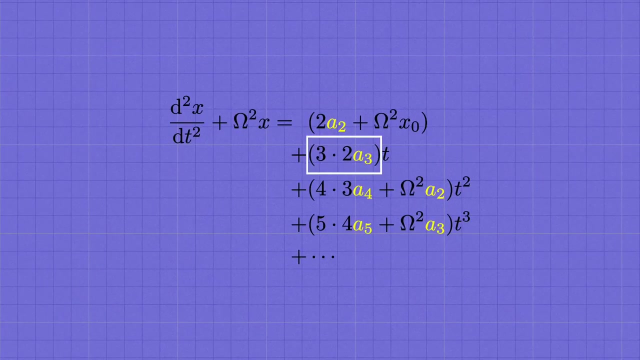 And the only way that can happen for every time t is if all the coefficients are separate and are inherently equal to zero. So the idea is to go term by term through the series and demand that each factor in parentheses is zero. Let's start with the odd terms. The coefficient of the 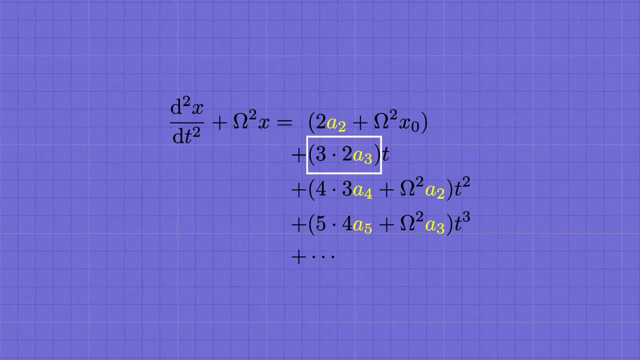 t term is three times two, a sub three. So for that to vanish, we need to choose a three equal to zero. Notice there's also an a three in the t cubed term, So I'll go ahead and erase that as well. 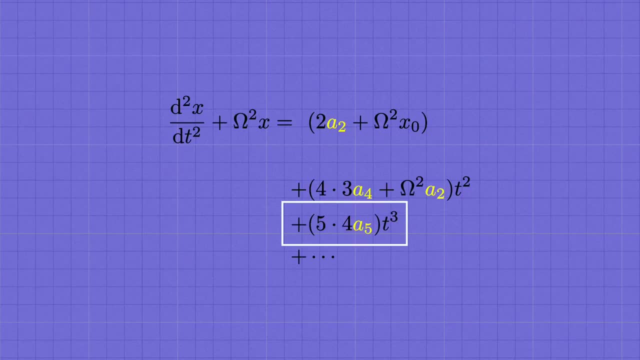 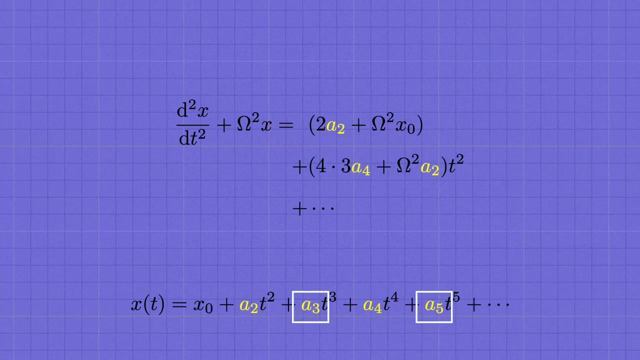 But now when we look at that t cubed term, its coefficient is just five times four, A sub five, And so for that to vanish, we'll also have to set a five equal to zero. The same thing is going to happen for all the odd terms. So we conclude that all the odd coefficients 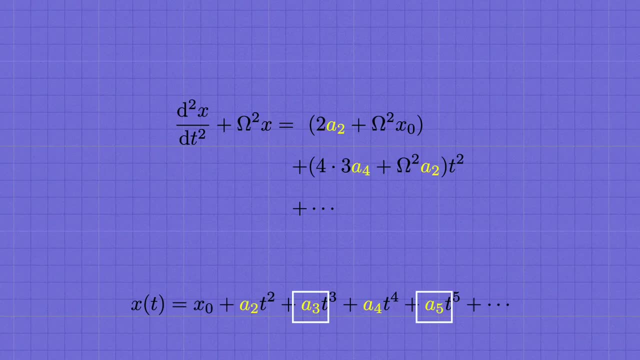 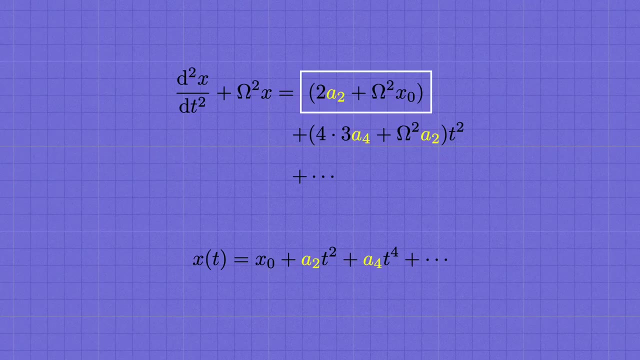 are equal to zero. That's already pretty nice, because it means we get to throw out half the terms in our expansion. So now let's move on to the even terms. The zeroth one says that two a two plus omega squared x zero is equal to zero, And so we can solve that for a sub two. 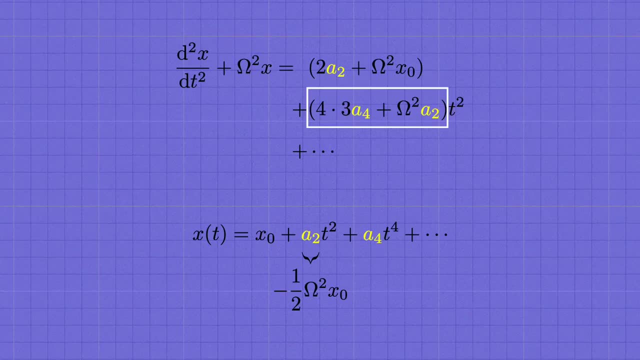 Next for the t squared term, we've got four times three, a four, plus omega squared a two and we set that equal to zero. Again, we can solve to get a sub four. Don't worry too much about that algebra. The point is, you can already see the pattern. 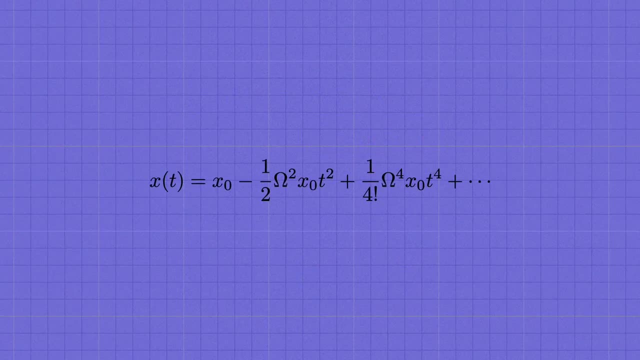 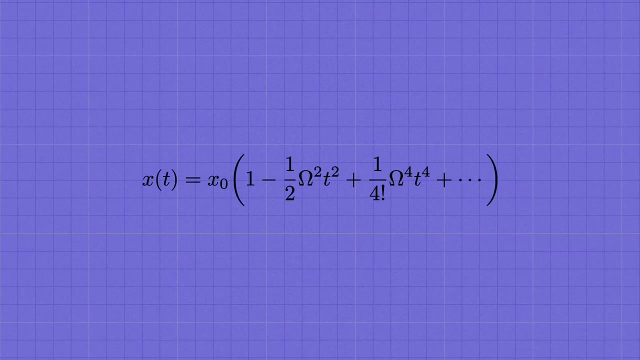 that's forming here. Here are the first few terms we're getting for our series solution. Does that look familiar at all? Let's simplify it a bit by pulling out the common factor of x- zero, And we can also put the omegas and the T's together like this. 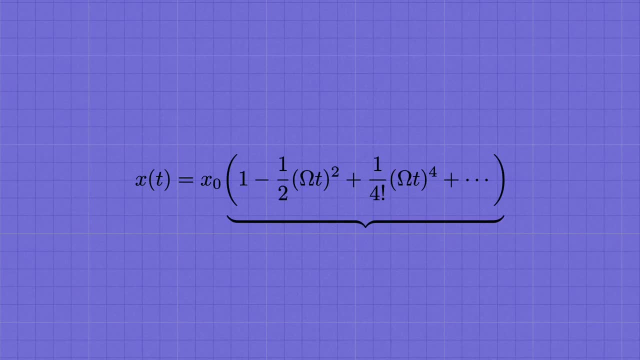 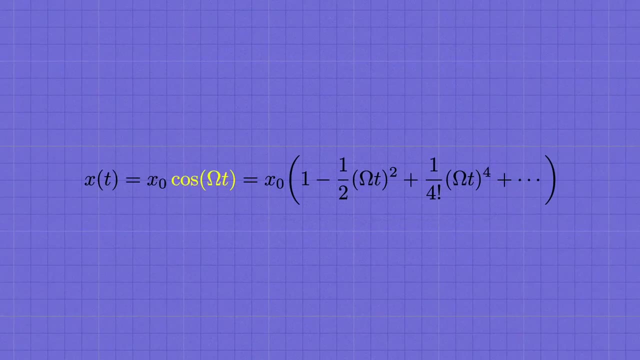 now Does this thing look like the Taylor series for any function that you know? That's right. The sum in parentheses is just the Taylor series for the cosine, And so, reassuringly, we've once again found that x of t equals x, zero cosine, omega t. 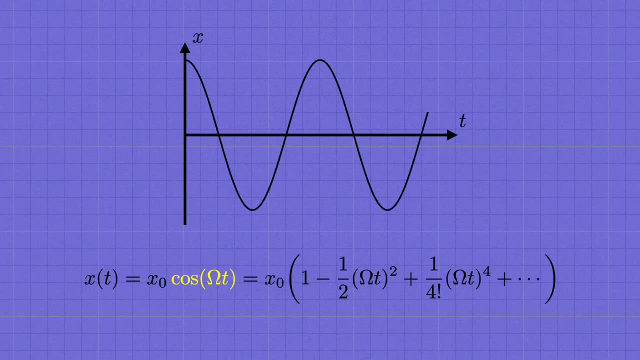 Like I mentioned, series expansions like this are an extremely versatile method for solving all kinds of differential equations. They don't always add up to a simple looking function like this, but that doesn't make them any less useful or valid as a solution to the equation, as long as you're looking at a point where the series converges. 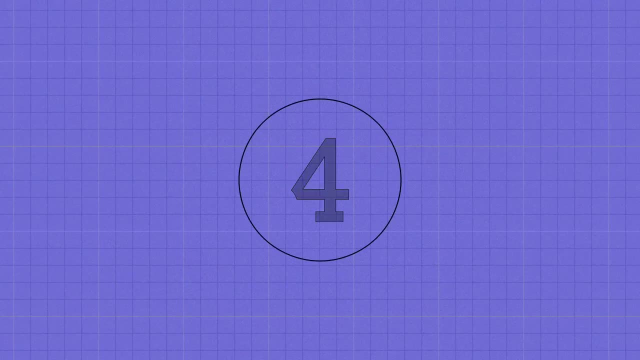 Okay, we're on a roll here. Let's keep it going with our next method: using an integral transform to solve a differential equation. We're definitely getting a little more advanced here, but this is really cool, so stick with me. There are lots of kinds of integral transforms. 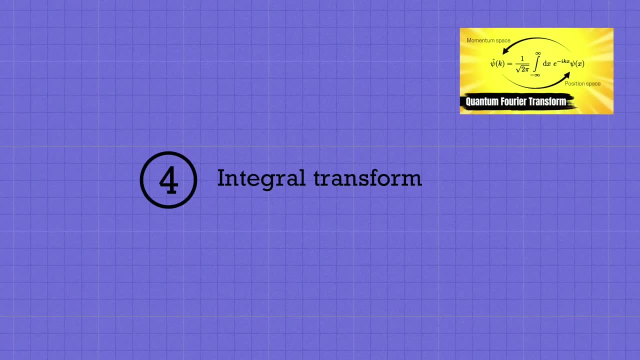 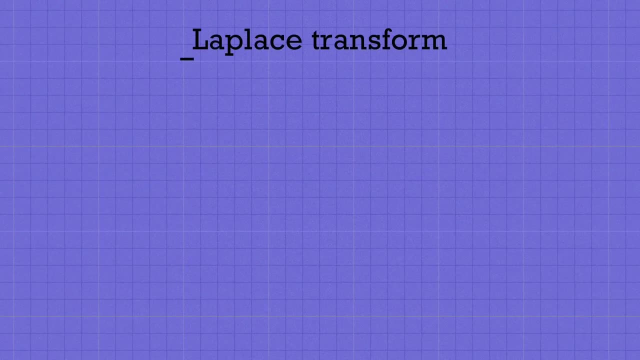 out there, including the Fourier transform, which my last video was actually all about, But the one that's most useful for solving the problem we're looking for is the integral transform, called the Laplace transform, And here's what it is, The Laplace transform. 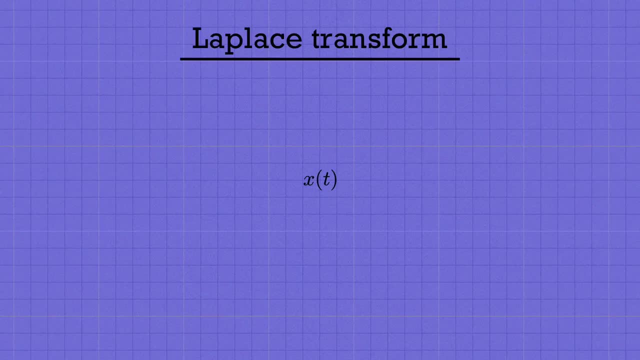 is an instruction to take our position. function x of t, multiply it by e to the minus st, with some new variable called s, and then integrate that over t from zero all the way to t equals infinity, And we'll call that x-hat of s. 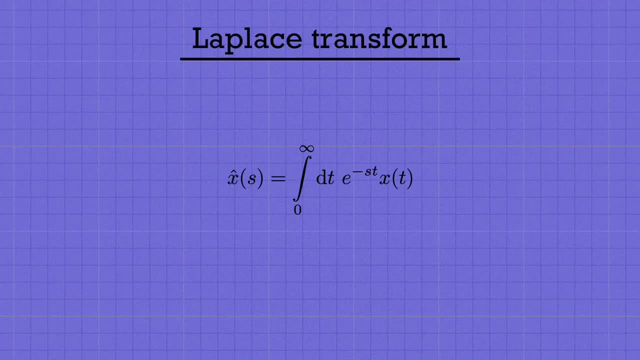 Okay well, that sounds like a funny thing to do, especially if you've never seen it before. But we'll see in a second that this transformation has a mass. Okay well, that sounds like a funny thing to do, especially if you've never seen it. before, But we'll see in a second that this transformation has a mass. Okay, well, that sounds like a funny thing to do, especially if you've never seen it before, But we'll see in a second that this transformation has a mass. 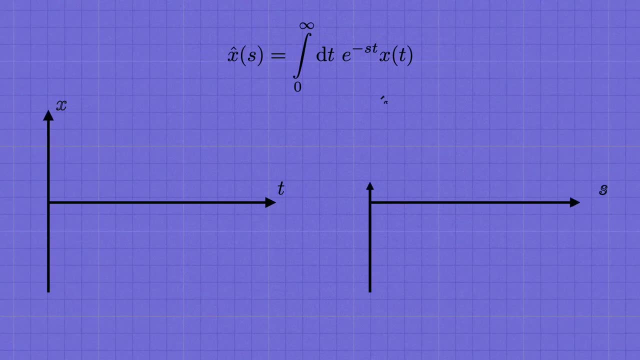 Okay. well, that sounds like a funny thing to do, especially if you've never seen it before, But we'll see in a second that this transformation has a mass. The way you should think about it, though, is that we have two spaces here: T-space. 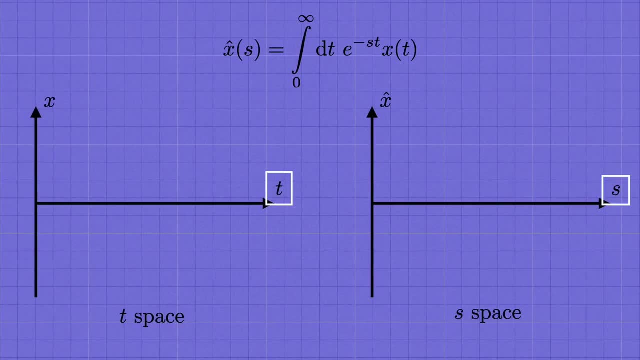 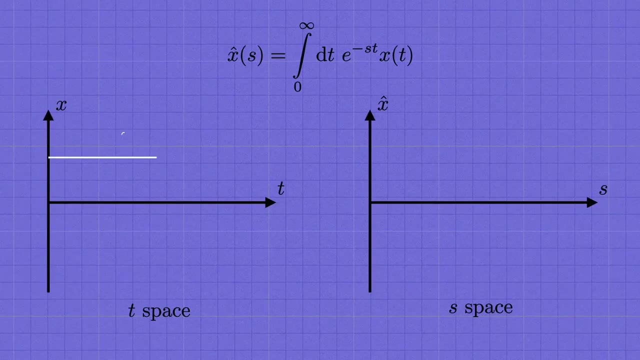 where our original function x of t, lives, and s-space where its Laplace transform lives x-hat of s. To give a couple of examples: if x of t were a constant, like say, x of t equals one, then it's just a horizontal line in t-space And you can show pretty easily. 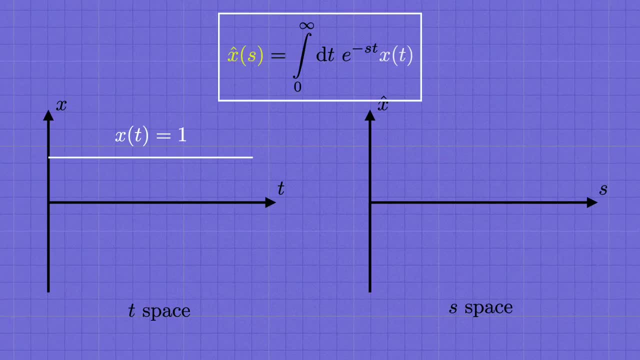 that it's Laplace transform in s-space obtained by doing this integral Or for our block on a spring. we found, and we're about to find again, that x of t equals x zero cosine omega t. It oscillates in t-space And in s-space its Laplace transform. 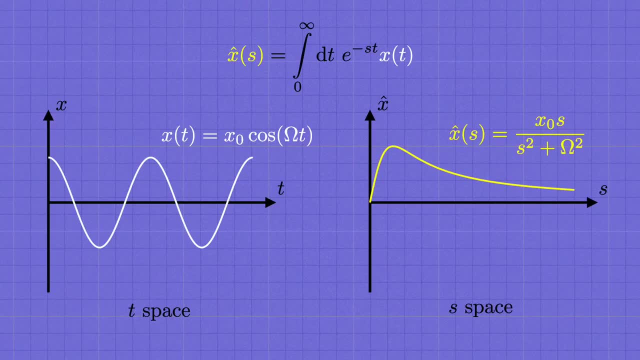 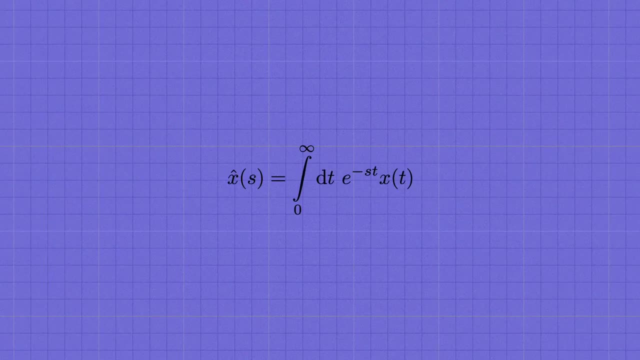 is a rational function: x zero times s divided by s squared plus omega squared. Alright, so we can do this integral to go from t-space to s-space. Big whoop. Why the heck would we want to do such a thing? How does it help us solve a differential? 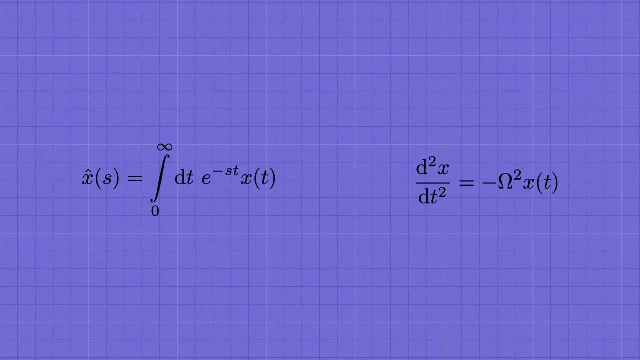 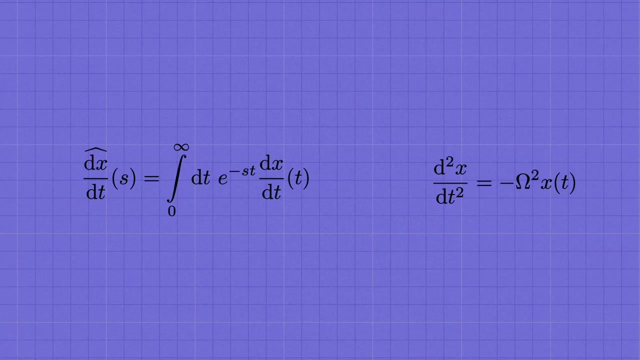 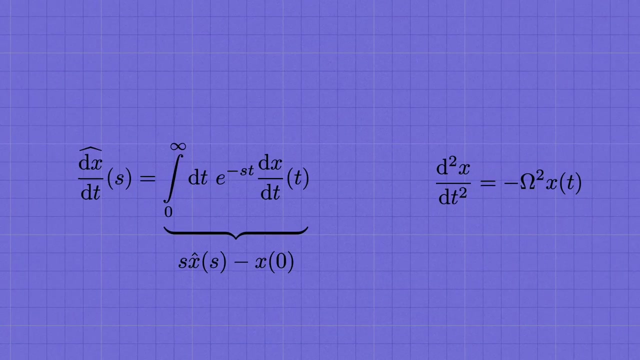 Well, a differential equation, like our harmonic oscillator. The reason is that the Laplace transform acts in a beautifully simple way on derivatives. When we take the transform of the derivative dx by dt, it turns into s times x-hat of s minus the initial position. 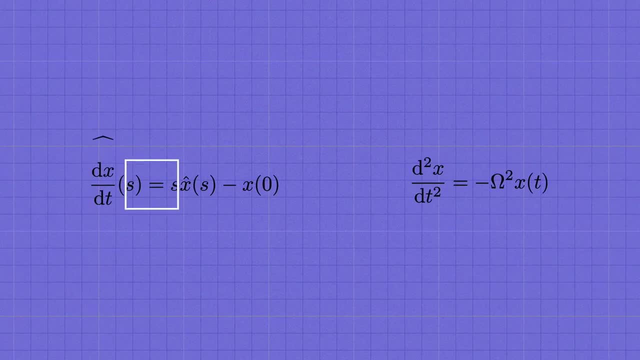 In other words, taking a derivative in t-space is the same as simply multiplying by s in s-space, up to a shift by x zero. And that follows just by using integration by parts of the Laplace transform integral. I'll show you how that works in the notes. 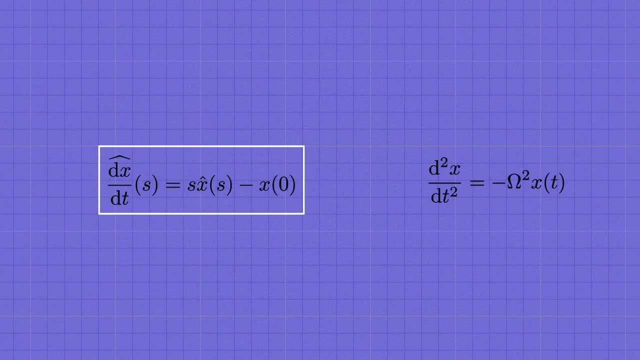 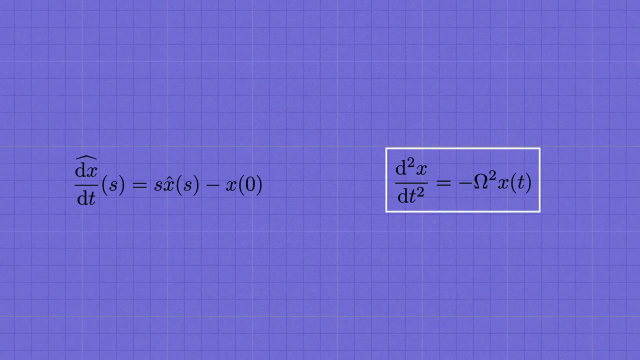 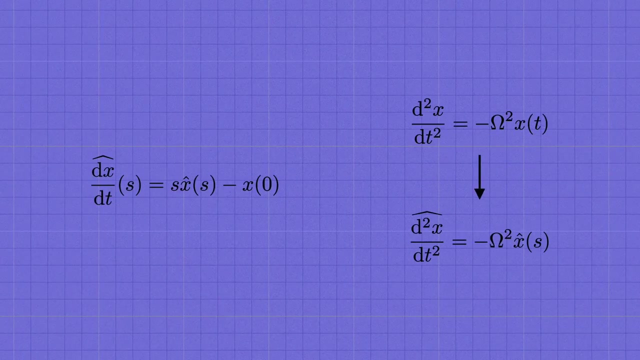 But the point is, because of this beautiful property, the Laplace transform can turn a differential equation for x of t into an algebraic equation for x-hat of s. Let's see how that works for our harmonic oscillator equation. We'll take the Laplace transform of both sides. 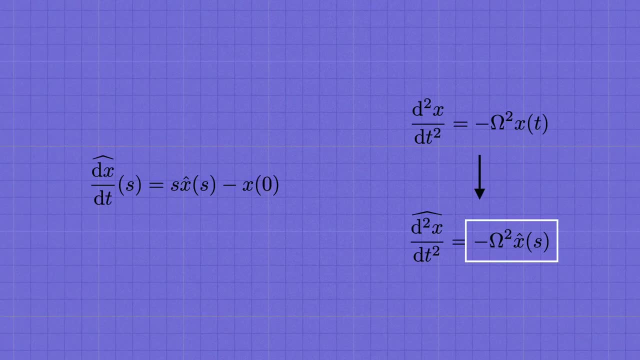 On the right, we just get that constant minus omega squared times the Laplace transform of x. On the left, we need to use our derivative rule twice in a row. If you work that out, you'll get s squared times x-hat minus s times the. 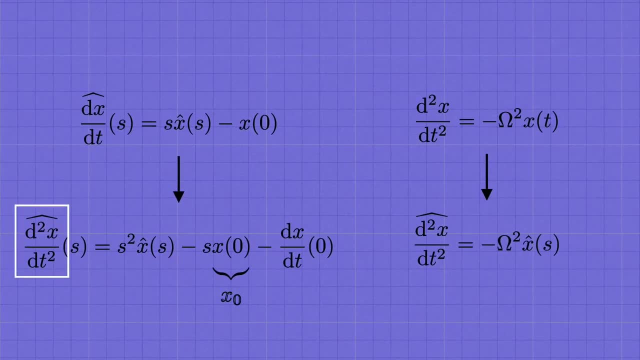 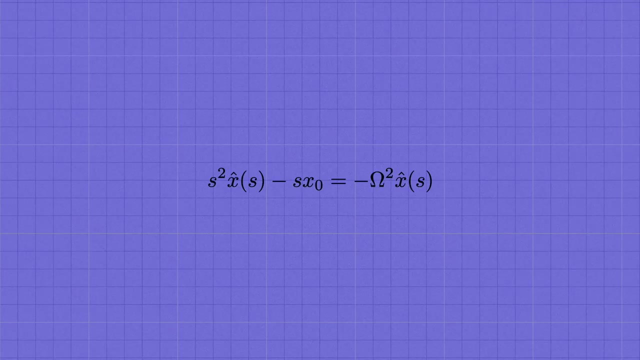 initial position minus the initial velocity. And if we plug in our initial conditions, we find that when we transform our differential equation to s-space, it becomes s squared times x-hat minus s x. zero equals minus omega squared x-hat. Like I promised there, 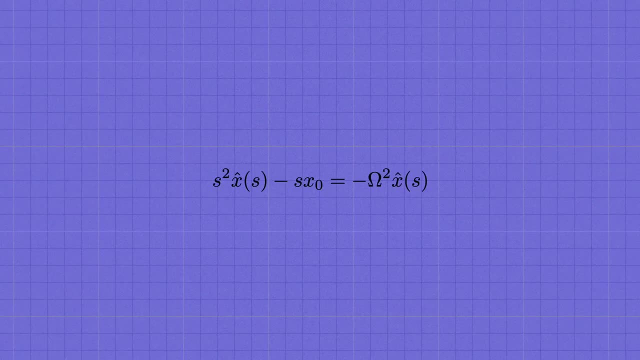 are no more derivatives. The Laplace transform took our differential equation for x of t and turned it into an algebraic equation for x-hat of s, And this equation is much easier to solve. Just move the x-hats over to the left and then divide out that factor. 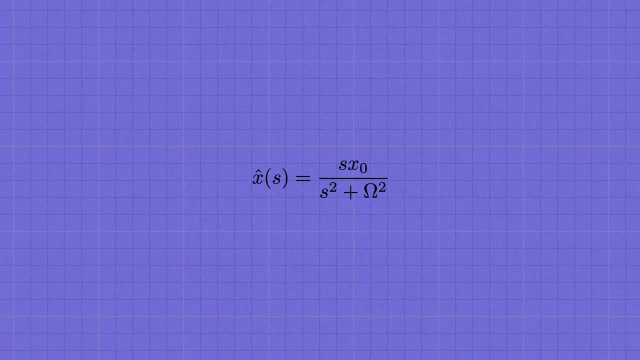 out front to get x-hat of s equals s x zero divided by s squared plus omega squared, And that's the solution to our problem in s-space. anyway, To finish the job, we just need to transform back to t-space. There's a general formula. 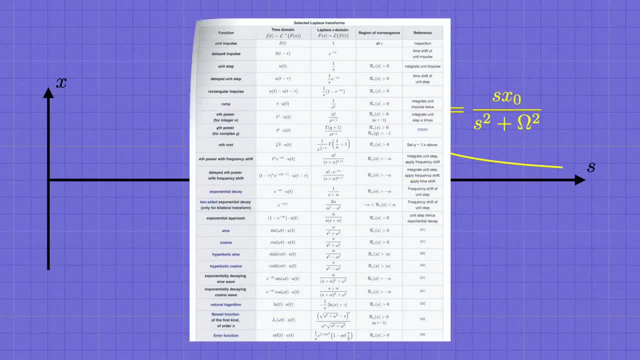 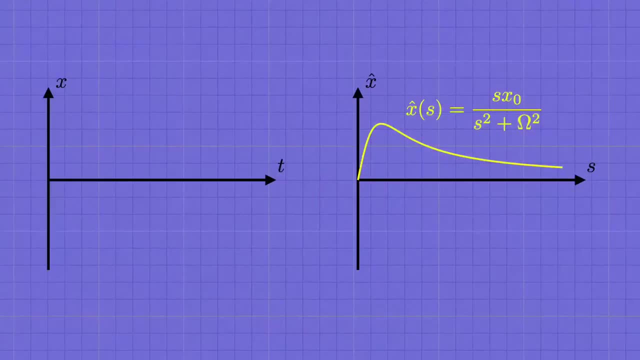 for doing that, but in practice it's often faster to just pull up a table of all the Laplace transforms- There's a nice one on Wikipedia- and find the one you're looking for. In fact, I already mentioned that this function is the Laplace transform of x zero. 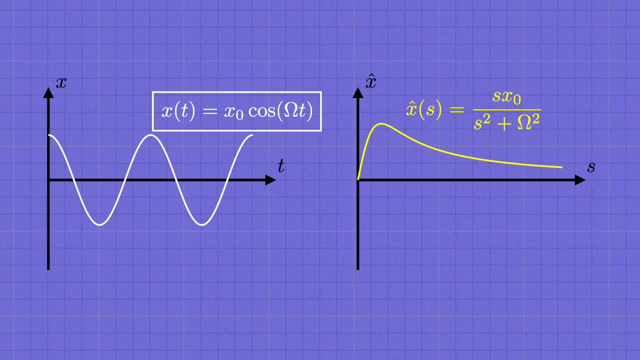 cosine omega t, And therefore that's the solution to our original equation once again. So that's method number four. Starting from a linear differential equation, take the Laplace transform to try to turn it into an algebraic equation which you can solve for x-hat And 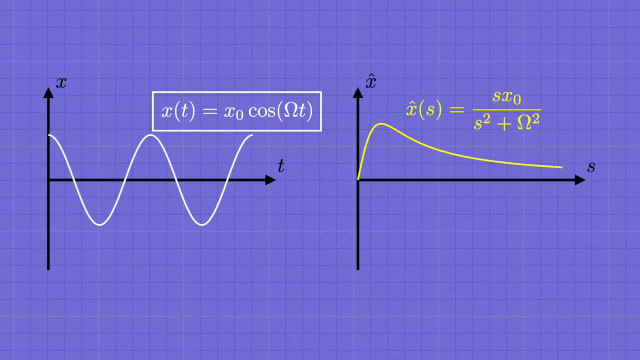 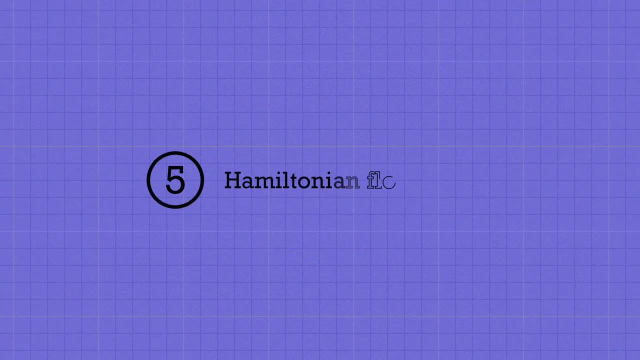 finally transform back to get your solution for x. Alright, we're in the homestretch now And I saved maybe the most fascinating of all of these for last Hamilton's equations and flows on face space. Let me show you how it. 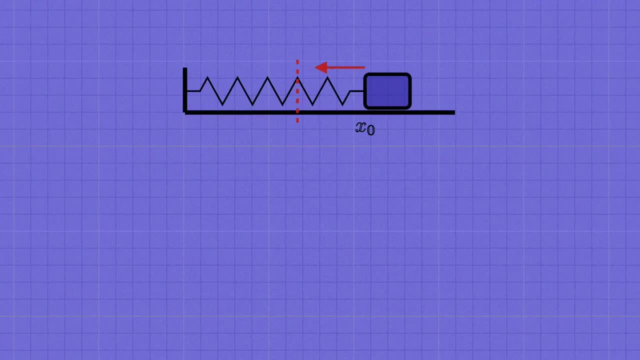 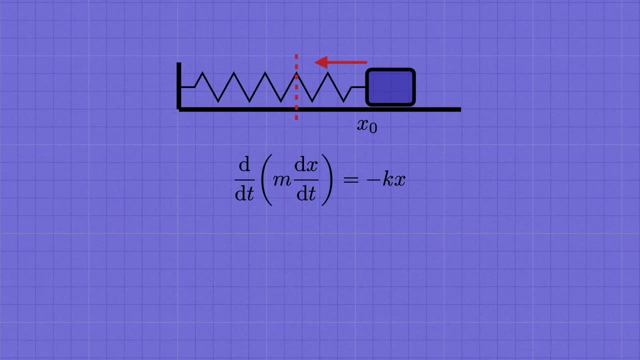 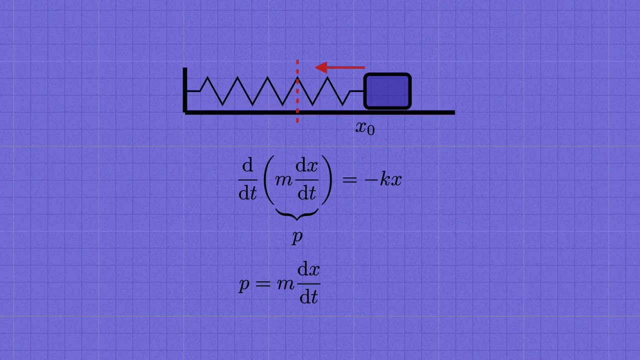 works. We started out with the f equals m-a equation for a block on a spring. Now notice that the left hand side is the same as the derivative of m times dx by dt, since m is a constant. In other words, it's the derivative of the momentum p. That's just Newton's second. 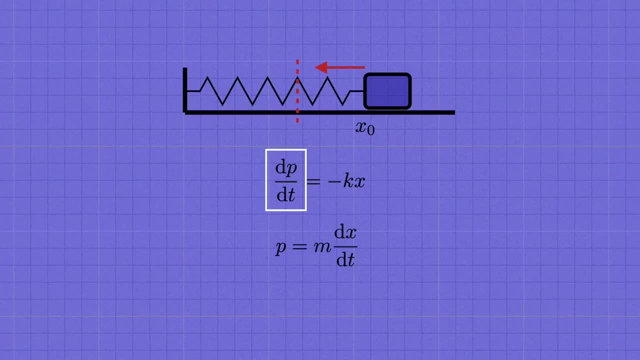 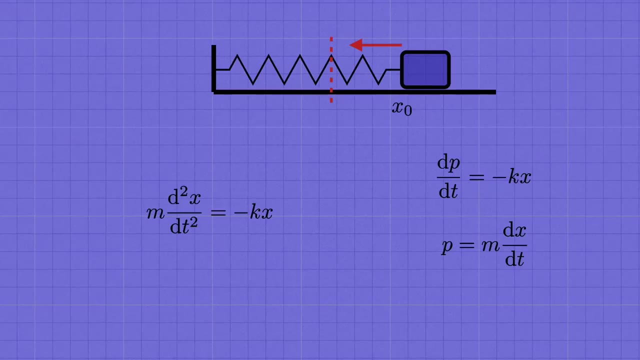 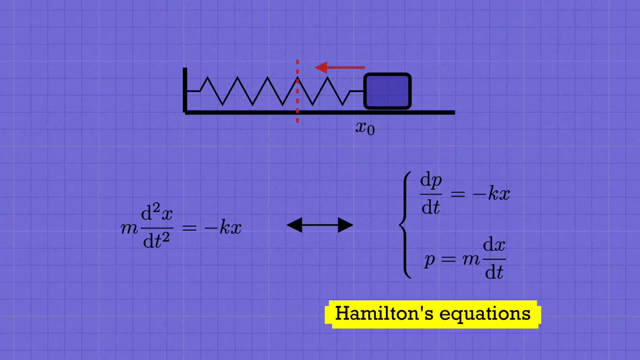 law. So we're looking for a solution for f equals m-kx and we'll use that for our first order equation. But mathematically, what that enables us to do is replace the single second order differential equation we started with with a pair of first order equations. These are called Hamilton's. 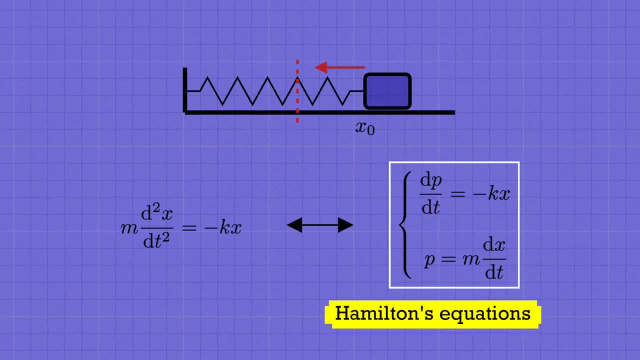 equations. I haven't done anything fancy. This pair of equations contains the exact same content as f equals m-a. All I've done is split it up into two pieces, But working with the first order equations has a couple of big advantages. One, it's 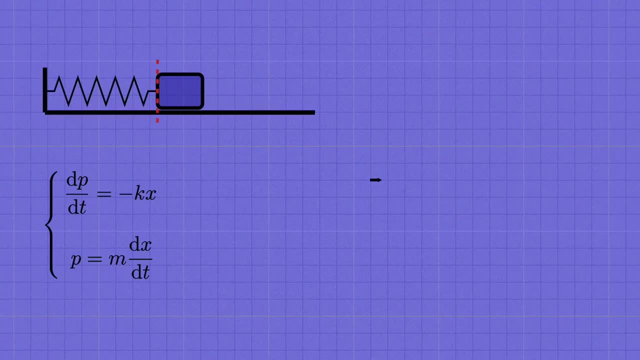 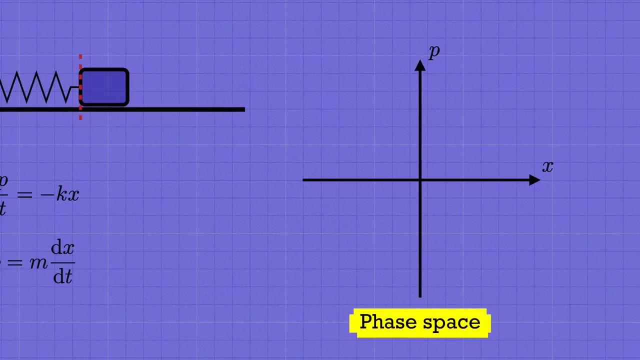 big advantages. To see why it's helpful, let's draw a picture with x on the horizontal axis and p on the vertical axis. This diagram is called the phase space, and each point in this plane tells us where the block is and what its momentum is, or, equivalently, its velocity at any given. 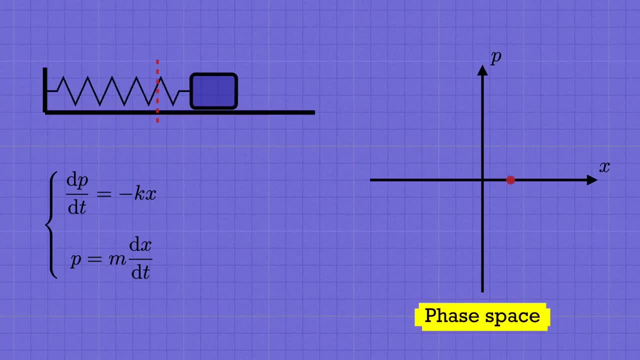 moment. So, for example, when we pull the block out to its initial position and then release it from rest, that initial state corresponds to this point here on the horizontal axis, where x equals x sub zero and p is equal to zero. After we let it go, the block is going to begin to move, and so these x. 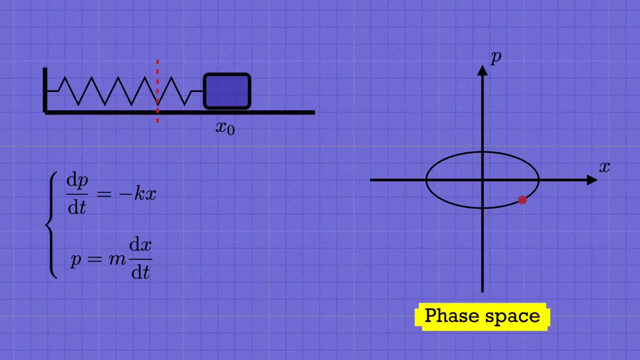 and p coordinates are going to change with time, So the point in this plane moves around with time and it traces out a curve called a flow, And flow really is a good name for it, because I want you to picture this plane like the surface of a pool of water, with some current running through it. 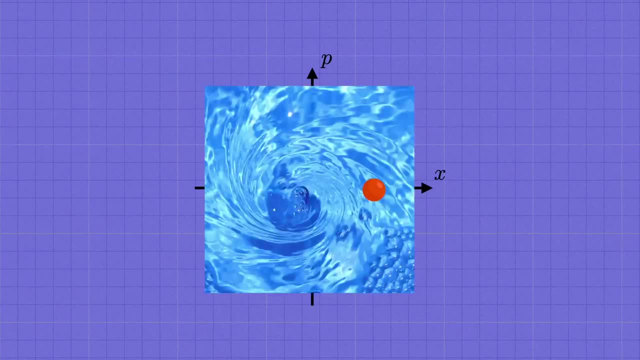 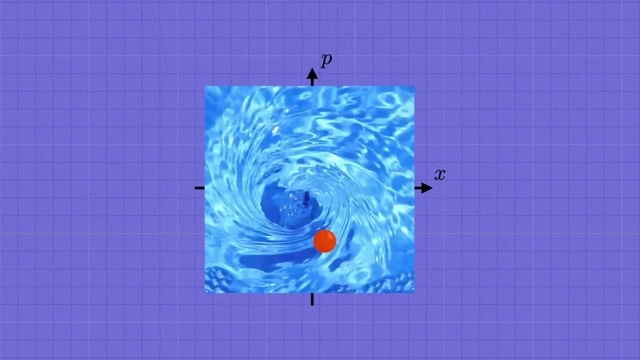 Then we take something like a ping pong ball, say, and set it down at the point for our initial conditions. Once we let it go, the current will carry the ball off, moving it around the surface of the water. The flow is the path that the ball follows through the water, But what determines the? 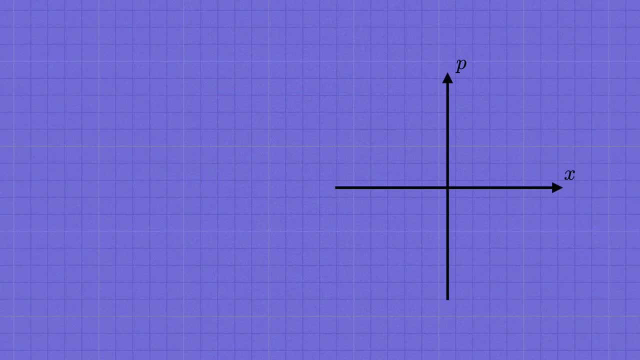 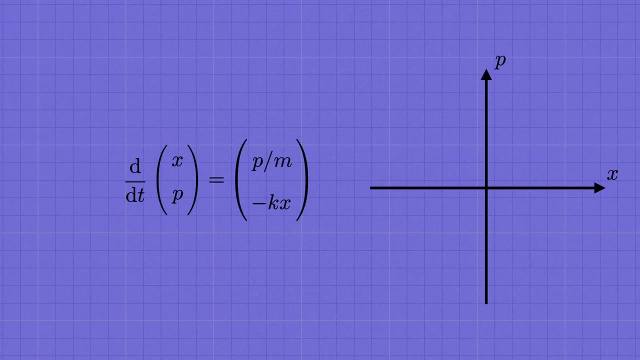 shape and strength of the current. that's telling the ball where to move Our differential equations. of course It's helpful to write the pair of them as a single vector equation. Again, x and p are the coordinates of the flow of the water. The flow is the path that the ball follows through the water. 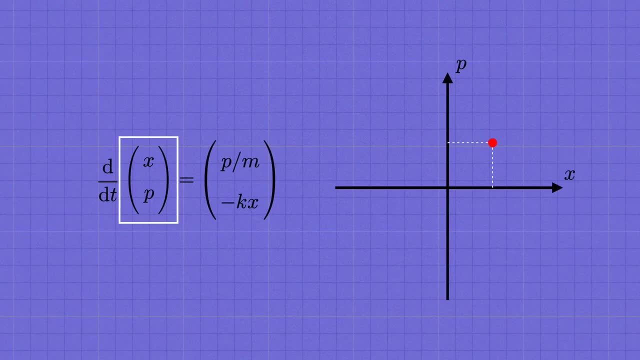 coordinates of the ping pong ball on the surface of the water, And so their time derivative is telling us the ball's velocity vector at each point on the surface Over here, at our initial point, x was positive and p was zero. Then the horizontal component of the velocity vector is zero and the vertical component 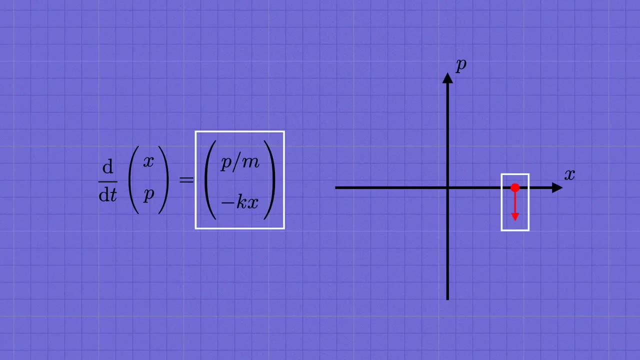 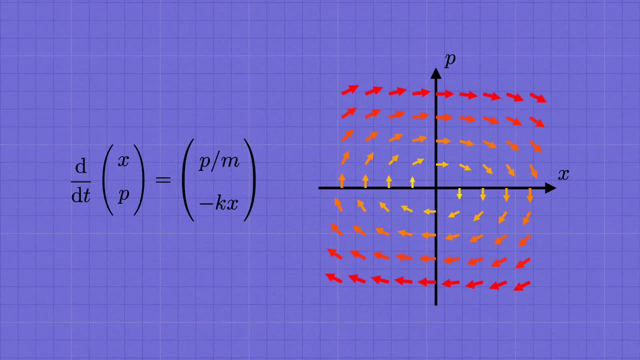 is negative. So the velocity of the imaginary ping pong ball points straight down at that point. Likewise, we can go to each point in this plane and draw this velocity vector. Those arrows are what tell us: the current that's swirling around the plane and what? 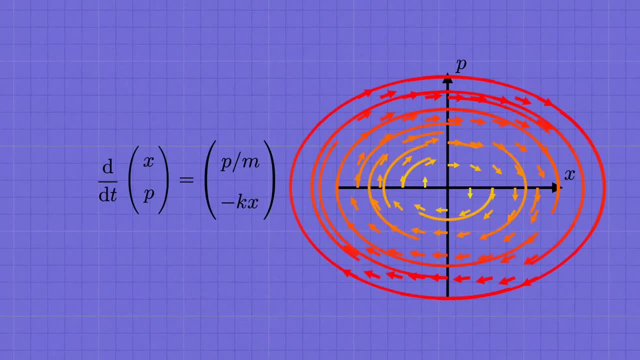 dictates how the ping pong ball will move. You can see that they're sort of swirling around the origin here. That's the equilibrium point, And I'm using the colors here to indicate how strong the current is. It's smallest for the yellow arrows near the middle and gets bigger for the red arrows. 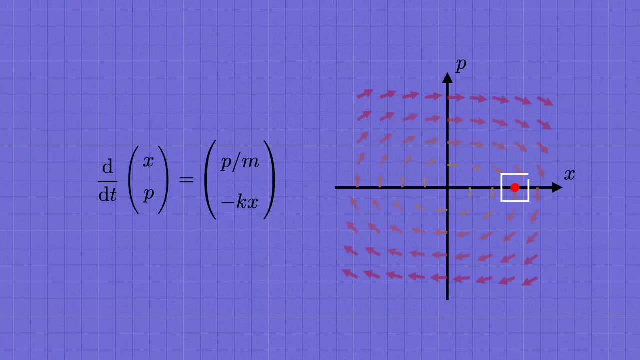 farther out By following those vectors. starting from our initial conditions, we see that the flow is an ellipse that wraps around the origin again and again, As the block oscillates back and forth around equilibrium. This is definitely a more abstract way of thinking about the solution to our differential 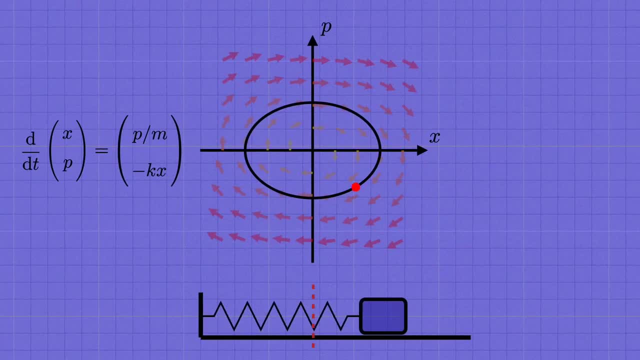 equation. Remember the physical system: here is the block sliding back and forth on this one-dimensional line, So obviously there isn't actually any pool of water or ping pong ball. Those are just useful mathematical constructs for picturing what's going on. But what this picture buys us is that we can very quickly understand what the motion of 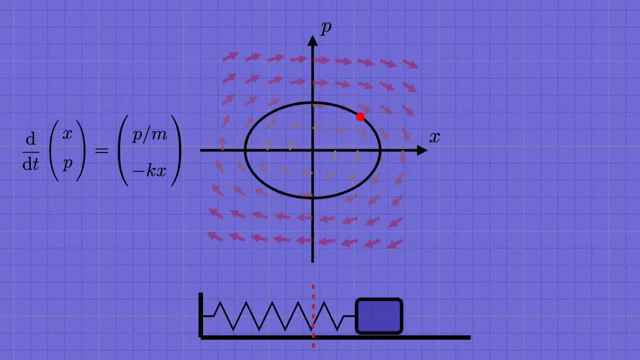 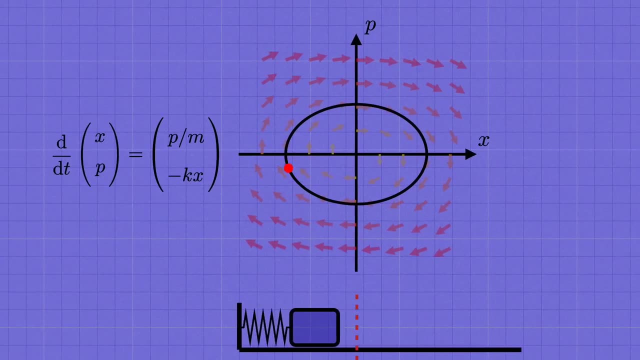 our system is going to look like Without solving any differential equations. all we need to do is draw the arrows at each point in phase space that we get from the right hand side of Hamilton's equations, Either by hand or, better yet, on a computer. 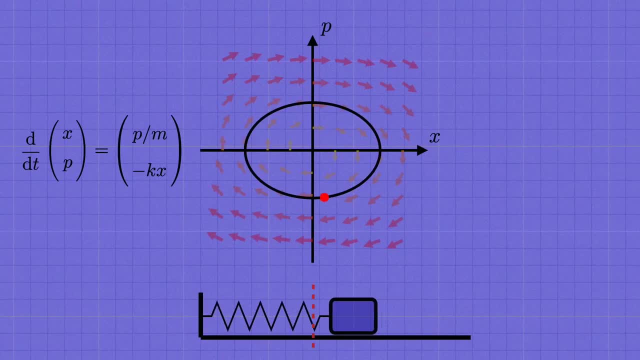 That's already an extremely useful way of thinking about differential equations, But Hamilton's formulation also gives us a really direct way of explicitly writing down the solution, At least for a linear equation like the harmonic oscillator. And that's the last thing I want to quickly sketch out for you. 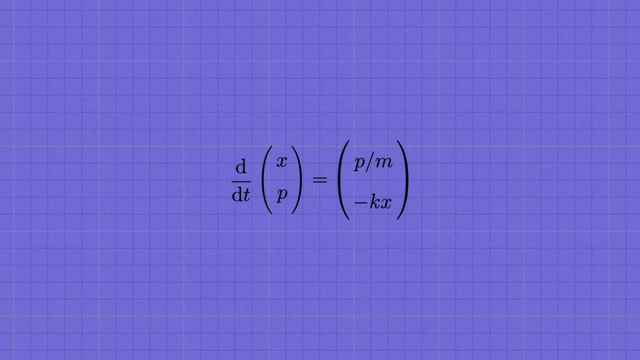 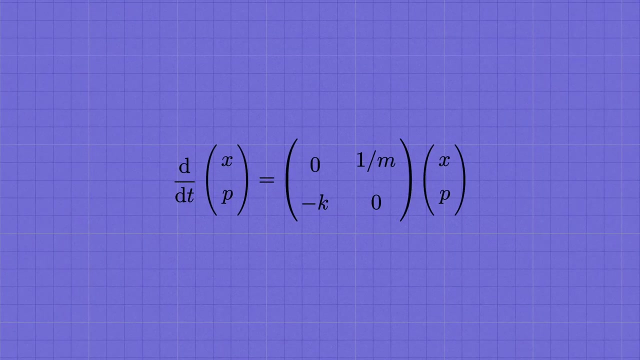 To see how it works, let's express Hamilton's equations as a matrix equation. This might look like we've made things more complicated, but hang on a second, we'll see how it pays off. Think about a simple differential equation like d by dt of z equals alpha times z for. 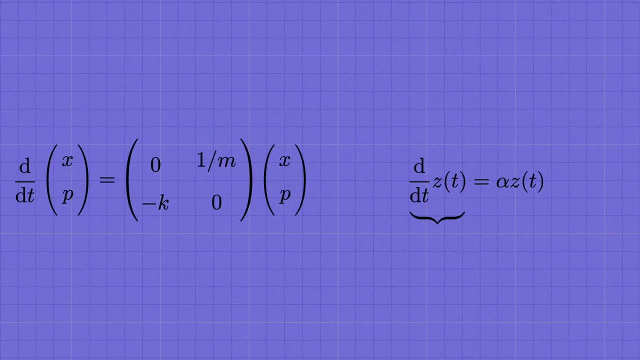 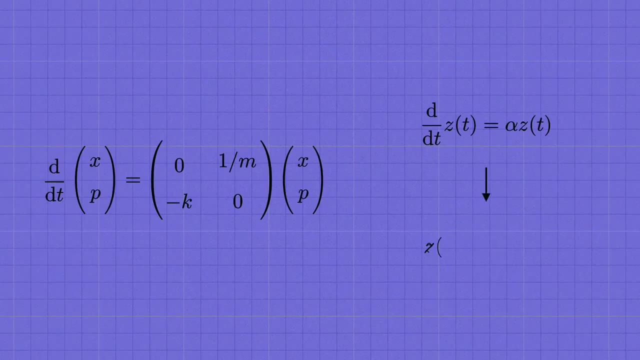 some constant alpha. This equation says that when we take the derivative of a function, z of t, we're supposed to get back z again times a number alpha. And the solution is simple: It's just e to the alpha t times z of t. 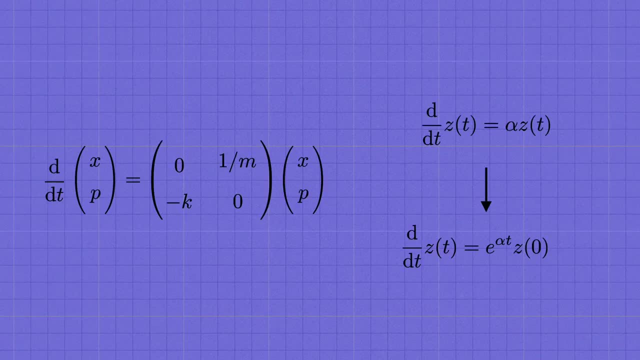 That's because the derivative of the exponential just turns back into itself, times a factor of alpha from the chain rule, And when you plug in t equals zero, you get that initial value z of zero. But notice that our matrix equation for the block on a spring is essentially of the same. 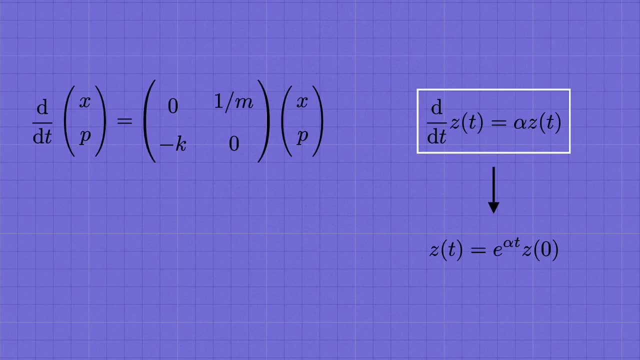 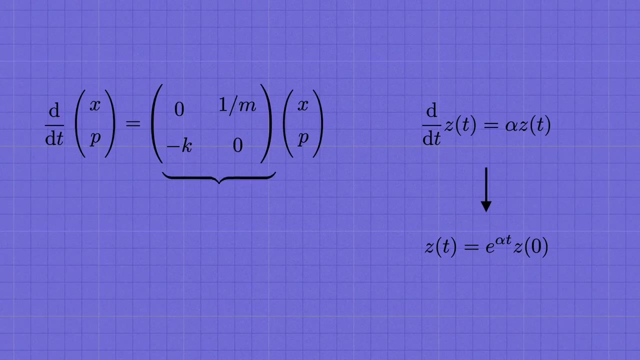 form only with vectors and matrices now instead of single numbers. It says that the derivative of the vector xp is equal to itself multiplied by a constant matrix, m, And the solution is simple. It's simple, It's just the matrix analog of our simple equation for z. 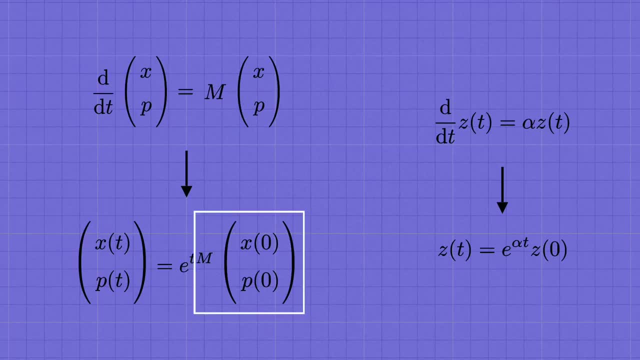 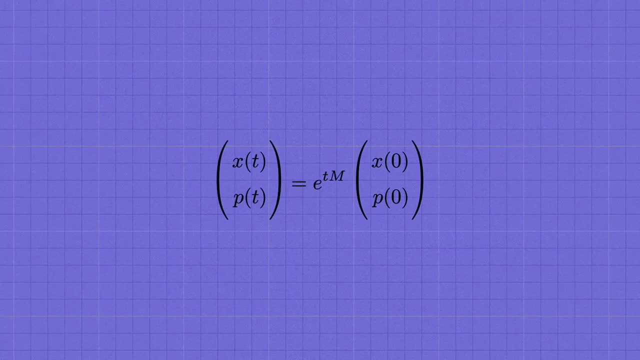 We take the initial vector, x of zero, p of zero and act on it with the matrix we get by exponentiating t times m. That looks reasonable, but of course we have to ask ourselves what it even means to take the exponential of a matrix here. 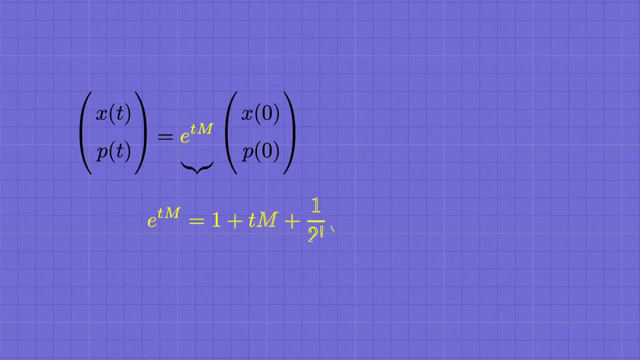 And it's defined by the usual Taylor series for e. We get one plus the thing in the exponent, plus half the thing squared, plus one over three factorial the thing cubed, and so on. That might look like a nasty thing to try to compute and it certainly can be in general. 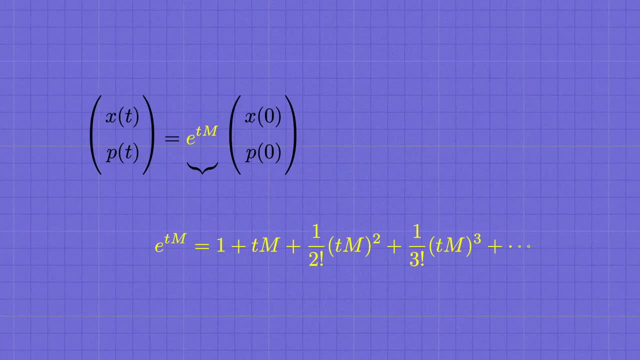 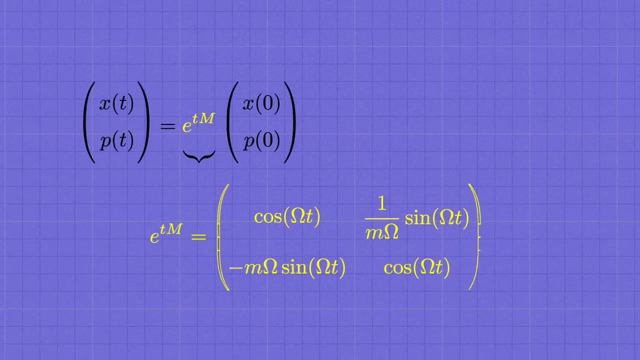 But for our matrix m in this problem the answer works out in a beautiful and simple way. Again, I'll show you how to get it step by step in the notes. But here's the result. We get cosine of omega t in the top left and bottom right and sine of omega t in the top. 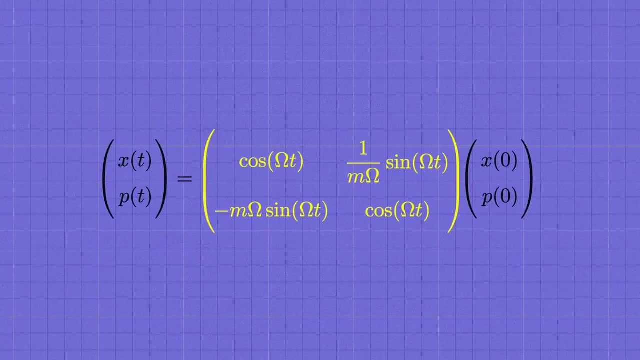